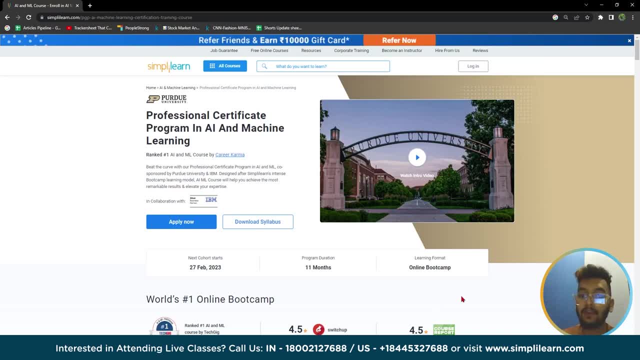 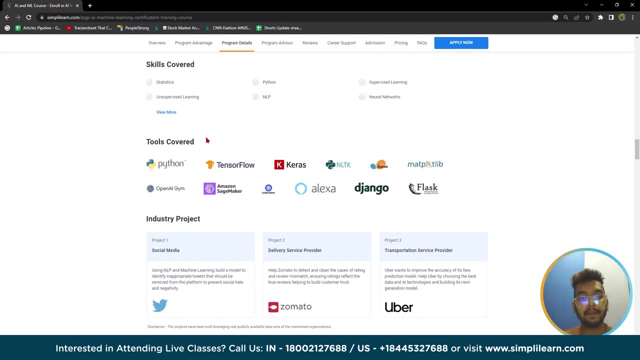 machine learning by 2023.. But you can beat the curve with a professional certificate program in AI and machine learning co-sponsored by Purdue University and IBM And that is designed after Simply Learn's intense boot camp learning model AI and ML certification course. So this course covers tools and techniques like Python, TensorFlow, Keras, NLTK and 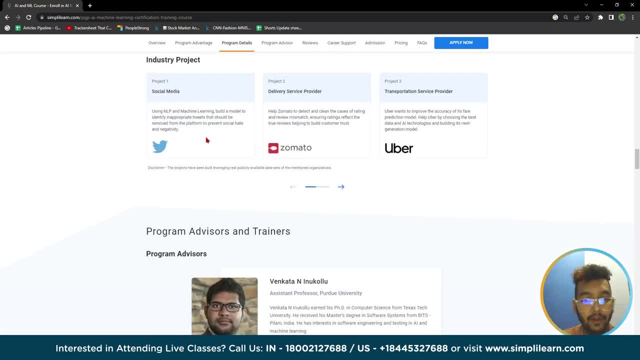 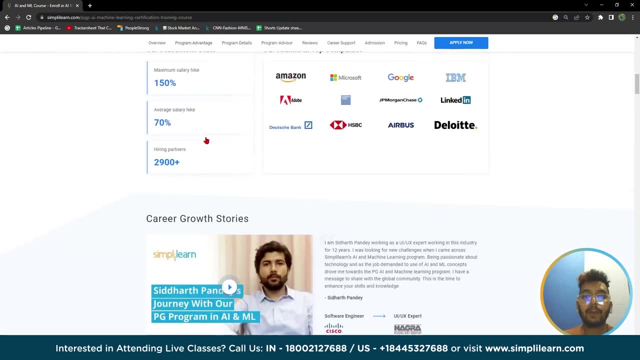 many more, along with industry projects like social media, Twitter, Zomato delivery service provider, Uber transportation service provider and many more amazing projects. So, choosing this course, can you get hired by renowned companies like Google, Amazon, LinkedIn and 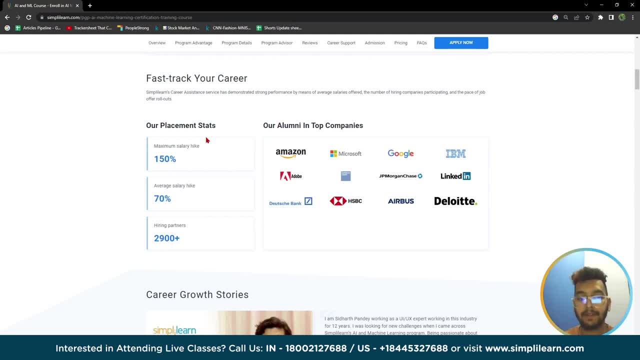 Adobe and an average salary hike of 70%. So what are you waiting for? Join the AI and ML professional certificate program and excel your career in AI and machine learning. So the link is in the description box below. Don't forget to check it out. 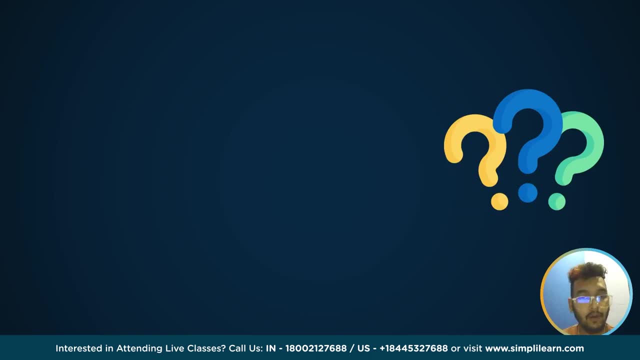 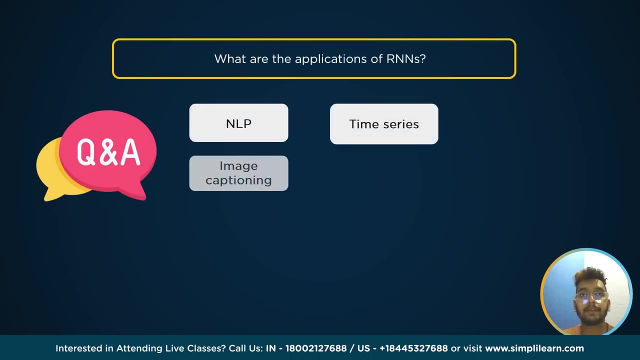 So before starting, let us have a simple question to brush up our knowledge. So question is: what are the application of RNN, Okay, NLP, time series, image captioning and all of the above? Please answer in the comment section below and we will update the correct. 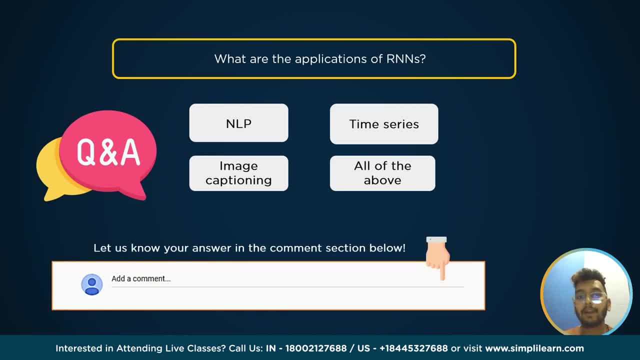 answer in the pinned comments, or you can pause this video, give it a thought and answer in the comment section. Before we move on to the programming part, let's discuss what RNN is and proceed further for the same. So what is RNN? 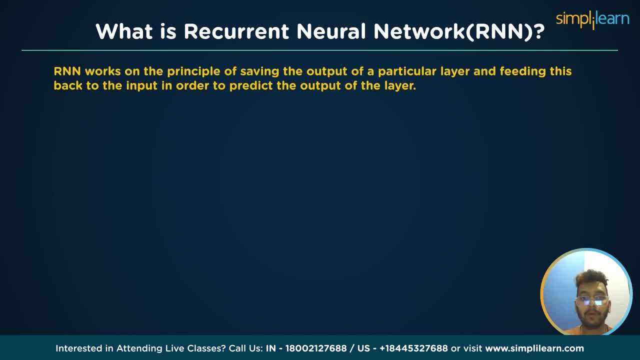 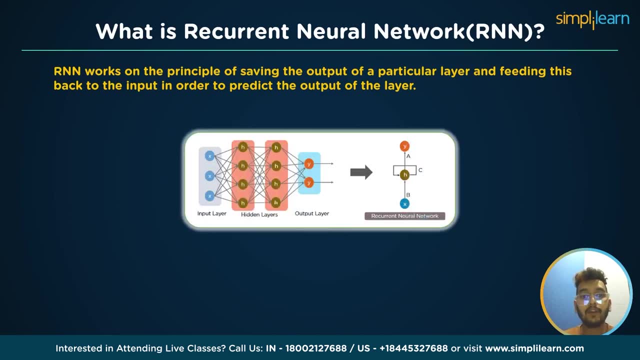 So RNN work on the principle of saving output on a particular layer and feeding this back to the input in order to predict the output of the layer. This is: how can convert a feed neural network into a recurrent neural network, The node in different layers of neural network. 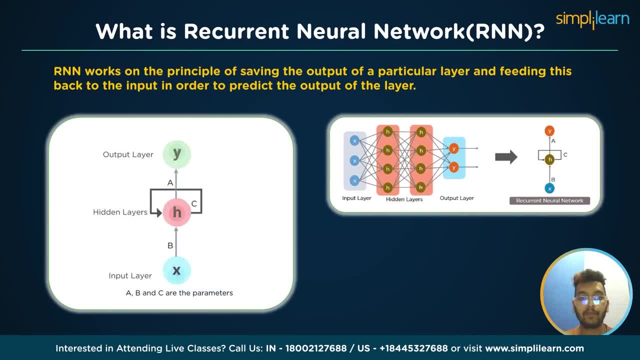 are compressed to form a single layer of recurrent neural network. A, B and C are the parameters of neural network. Now that you understand what RNN is, let's look at the way. why RNN. Okay, So why RNN? 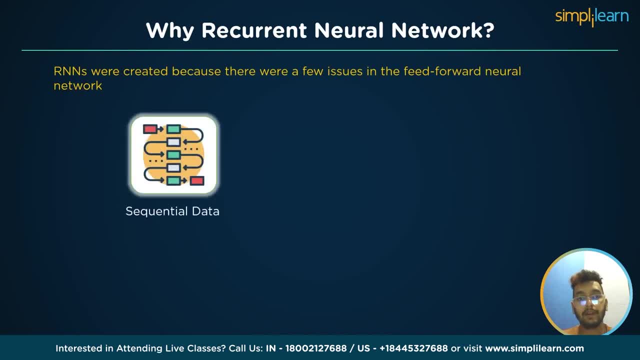 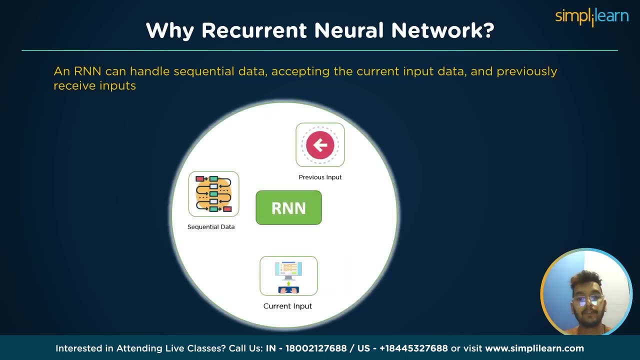 Well, the reason is because there are few issues in the feed forward. neural network Cannot handle sequential data, considers only the current input, cannot memorize previous input. Okay, So the solution of these issues is RNN And RNN can handle sequential data, accepting the current input data and previously received. 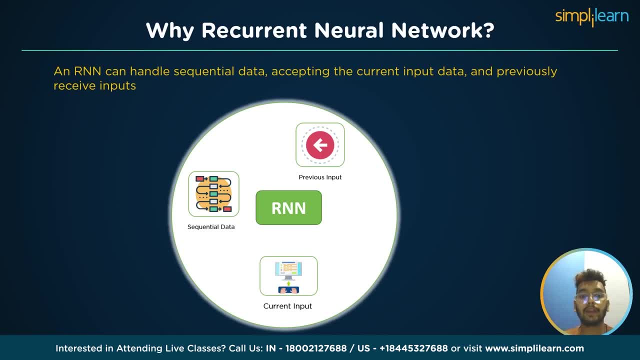 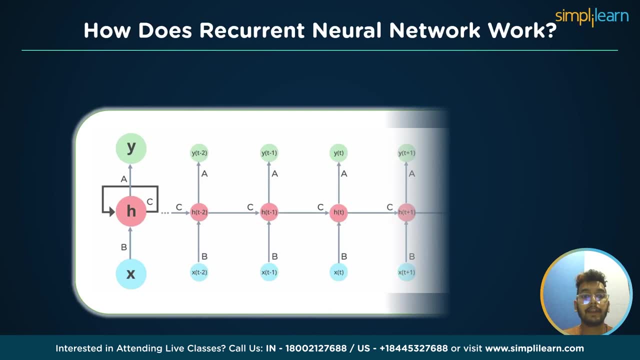 input data So RNN can memorize previous input due to their internal memory. So, moving forward, let's see how does RNN networks work? Okay, So the input layer X, Okay, to the neural network and process it and passes it into the middle layer. 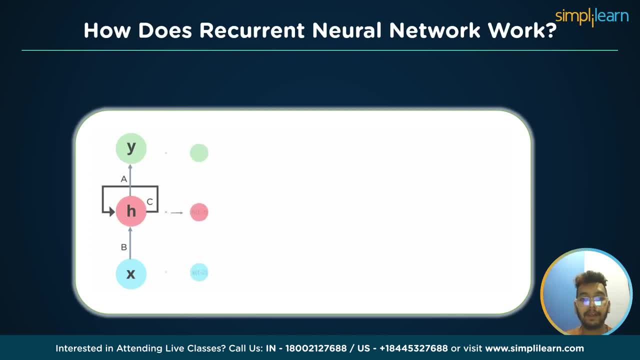 The middle layer H can consist of multiple hidden layers, each with its own activation, function and weight and biases. If you have a neural network where the various parameters of different hidden layers are not affected by the previous layer, ie the neural network does not have the memory, then 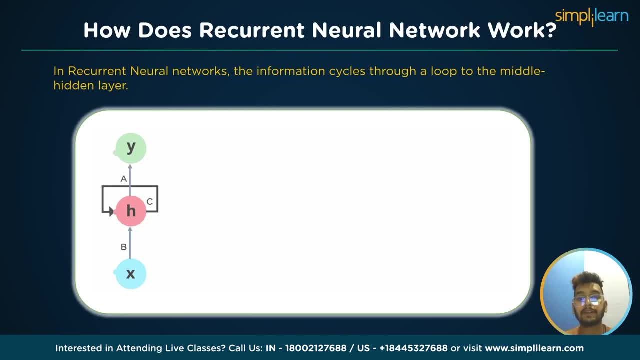 you can use RNN, So the RNN will standardize the different activation function and weights and biases so that each hidden layer has the same parameter. Then, instead of creating multiple hidden layers, it will create 1N loop over it as many times. 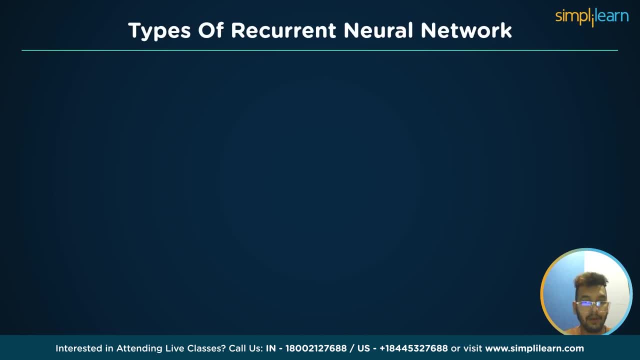 it has required. So, moving forward, let's see types of RNN. So there are four types of RNN: one-to-one, one-to-many, many-to-many and many-to-one. So let's see one-to-one RNN. 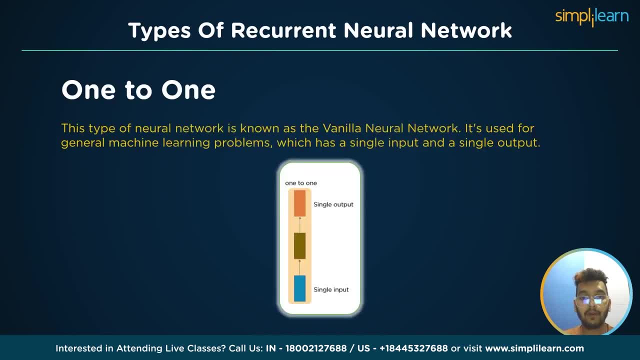 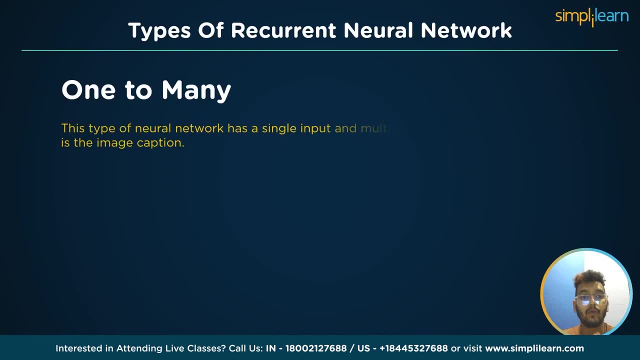 So this type of neural network is known as the Vanilla Neural Network. It is used for neural networks. It is used for general machine learning problem, which has a single input and a single output. Now see one-to-many RNN. This type of neural network has a single input and multiple outputs. 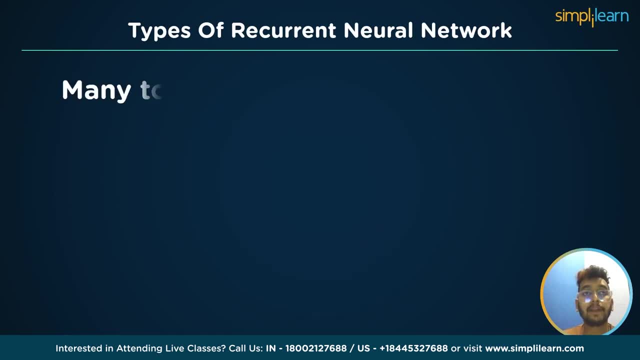 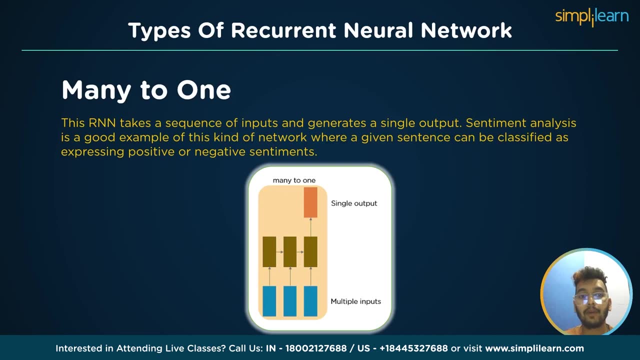 An example of this is an image captioning. Now let's see many-to-one RNN. This RNN take a sequence of input and generates a single output. Sentiment analysis is a good example of this kind of neural network, where a given sentence. 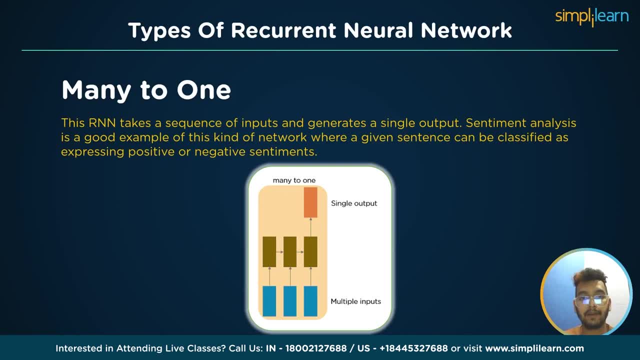 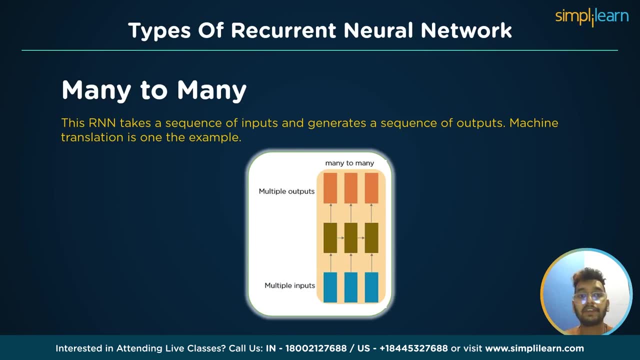 can be classified as expressing positive or negative sentiment, And the last one is many-to-many. This RNN takes a sequence of inputs and generates a sequence of outputs. Machine translation is one of the examples. So, moving forward, let's see application of recurrent neural network. 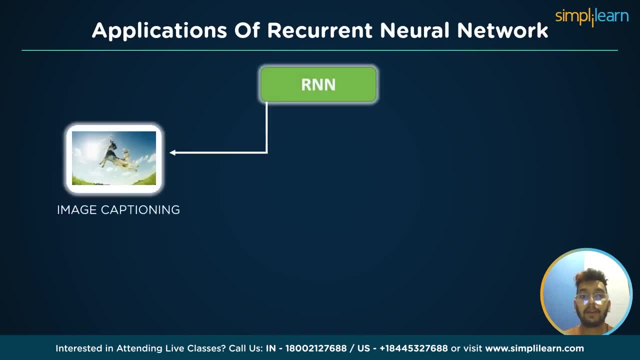 First one is image captioning. RNNs are used to caption an image by analyzing the activities present. The second one is time series prediction. Any time series problem, like predicting the prices of stocks in a particular month, can be solved using RNN. 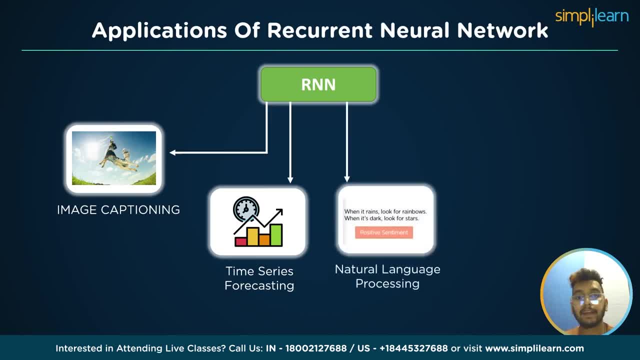 And the third one is time series prediction. The third one is natural language processing. Text mining and sentiment analysis can be carried out using RNN for NLP, natural language processing. The fourth one is machine translation. Given an input in one language, RNNs can be used to translate the input into different. 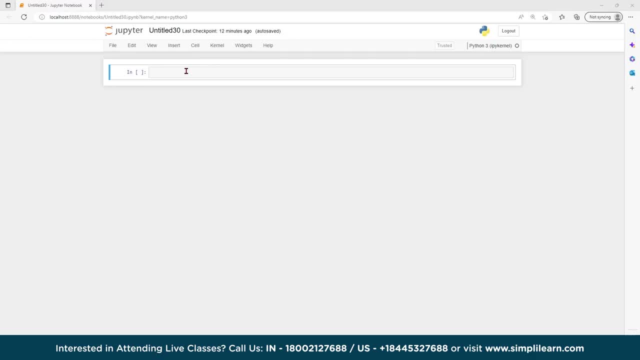 language as output. So now let's move to the programming part. First we will import some libraries, major libraries. for the first we will import for the data frame. So I will write import. So I will write import. Pandas is a software library written for the Python programming language for data manipulation. 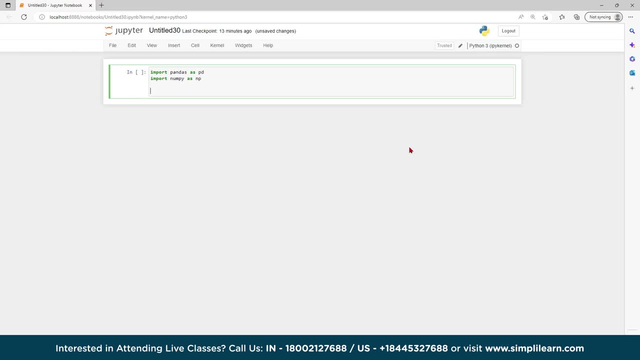 and analysis. In particular, it offers a data structure and operations for manipulating numerical tables and the time series, And this NumPy. NumPy is a library for the Python programming language, adding support to four large multi-tablet libraries, So it is a library for multi-dimensional array and matrices. along with the large collection, 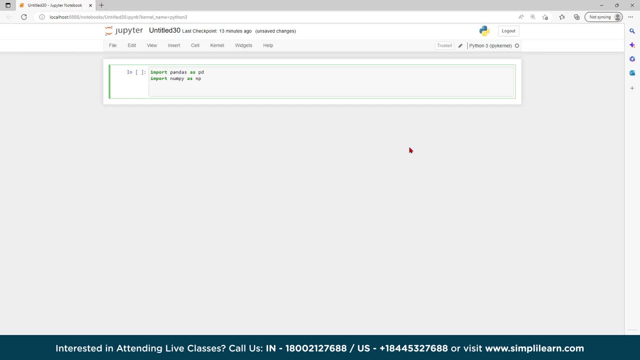 of high level mathematical function to operate on these arrays. OK, So for plotting we will import some libraries like seaborn as NS. This is nothing, just a sort form of we don't have to write again and again: seaborn, seaborn, We can write SNS. 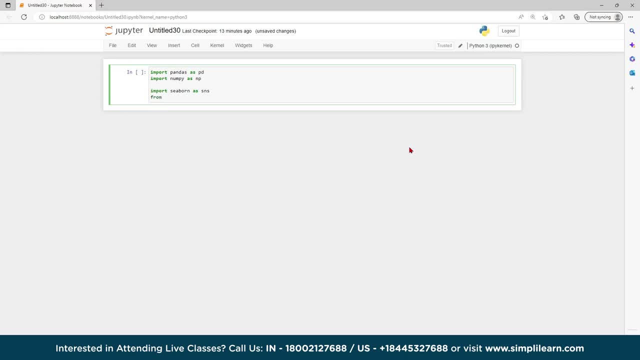 So then another one from SNS. OK, Nice, word cloud quote. word cloud quote. matplotlib dot, pyplot as plt. okay, so seaborn is a library that uses matplotlib underneath to plot graphs. it will be used to visualize zandam distribution and the word cloud is a visual representation of words. cloud creators are used to highlight. 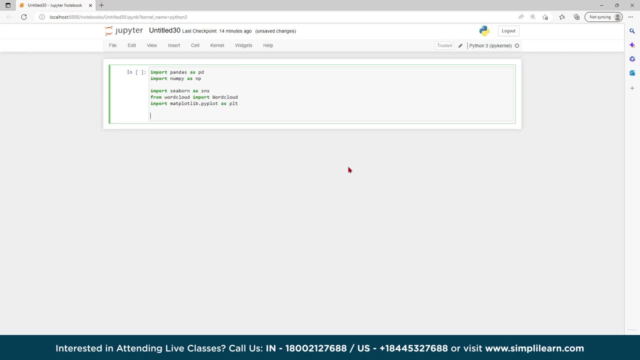 popular words and phrases based on frequency and relevance. they provide you with quick and simple visual insights that can lead to more in-depth analysis. and this matplotlib. matplotlib is a plotting library for the python programming language and its numerical mathematical extension number. it provides an object oriented api for embedding plots into application using general purpose ui. 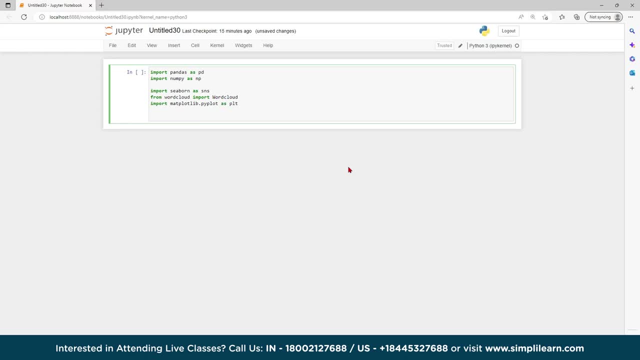 okay, like tinker wx, python, qt or gtk. so let's import some nltk natural language toolkit. so i will write: import nltk. okay. from nltk dot stem import word net nematizer. and from nltk dot corpus import stop words. then from nltk dot tokenize code word tokenize. 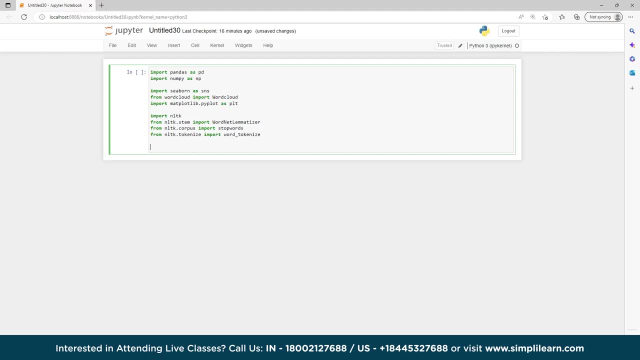 nltk, the natural language toolkit, or more commonly nltk, is a suite of libraries and programs for symbolic and statistical natural language processing for english written and python programming language, and this is stop words. stop words are words that are so common they are basically ignored by typical tokenizers, and this word tokenize is a function in python that 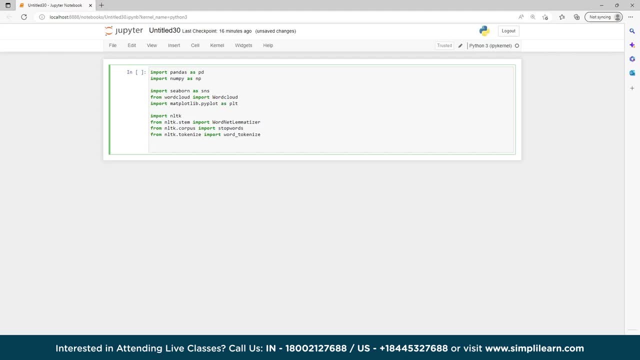 splits a given sentence into words using the nltk library- okay, so let's import some scikit-learn library. so for that i will write: from sklearn dot model selection- import- train test: okay. then from sklearn dot feature extraction selection: import- train test: okay. or text import: F ID vectorizers. 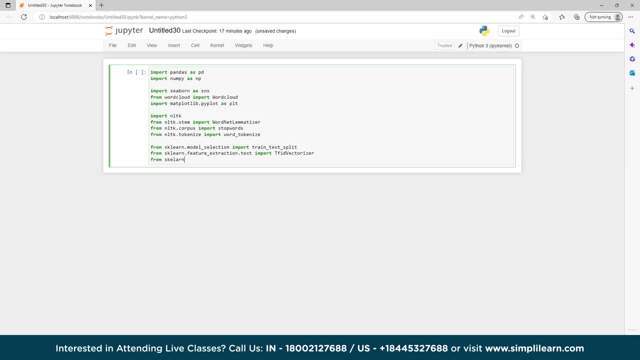 then from a skill on dot mattresses, metrics, import, confusion, metric you classification. okay. so second learn is a free source software machine learning library for Python programming language. it features various classification, regression and clustering algorithms, including support vector machine learning, logistic regression and many others like random forest classifier and this. 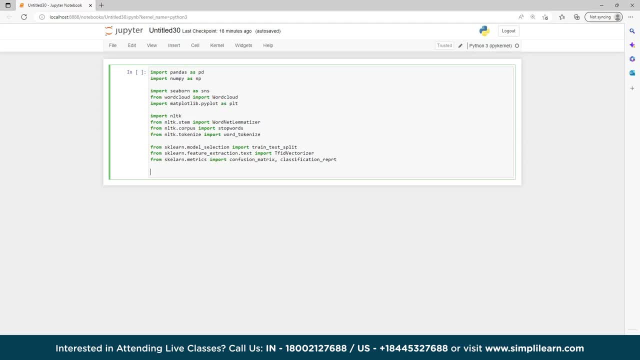 trigger-free is the following: and this trigger-free is the following: test split method is used to split our data into train and test set. first, we need to divide our data into features like x and y labels, and this tf id vectorizer converts a collection of raw. 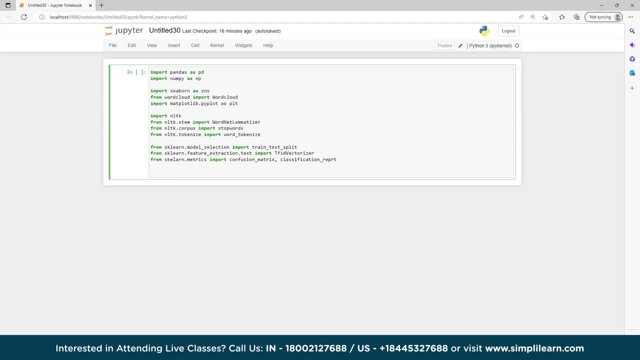 documents into a matrix of tf or idf features the fast text on what to vectorizer what, embedding python implementation and this confusion matrix. a confusion matrix is a table that is used to define the performance of a classification algorithm. okay, then we'll import some libraries like from sk learn dot linear model. 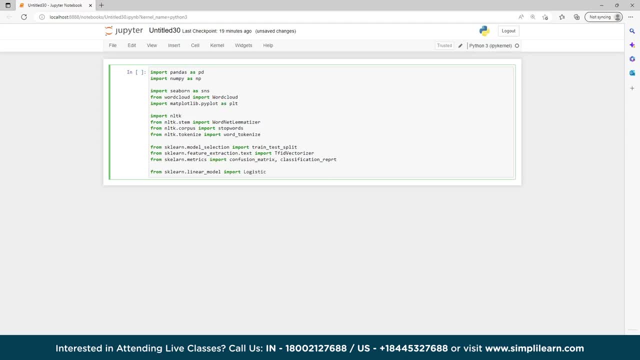 code: logistic regression. so then from ilan pm port, then from ilan symbol port: random forest classifier: okay, then from sk learn dot name base port, bernoulli base: okay. so let's say we know that usually everything is correct. so logistic regression estimates the probability of an event occurring, such as voted or didn't vote, based on a given dataset of the. 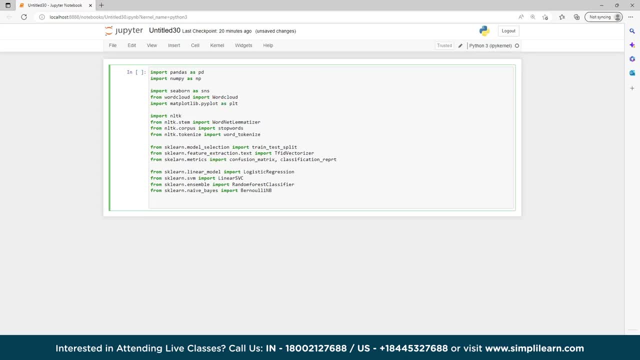 independent variable that attempts to find a hyperplane to maximize the distance between classified samples, and this random forest classifier creates a set of decision trees from a randomly selected subset of the training set. and this Bernoulli and we Bernoulli name base is a part of the name base family. it is: 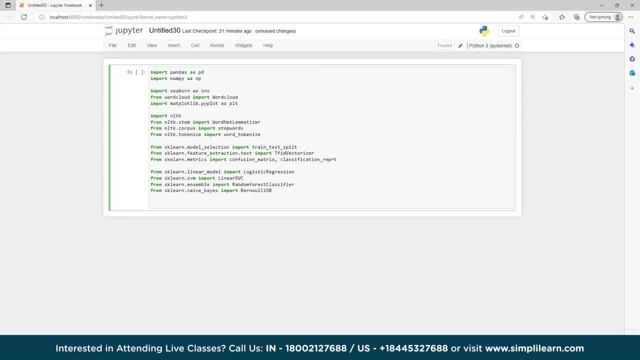 based on Bernoulli distribution and accept only binary values, that is, 0 or 1.. so let's import some tensorflow. so import tensorflow dot, compact, dot, v2 and then import tensorflow data sets as tfds. so tensorflow is a free and open source library for machine learning and 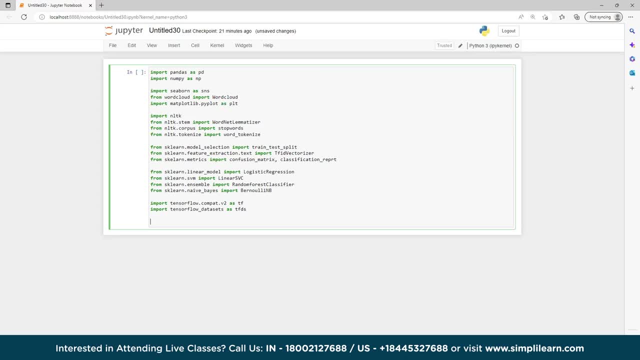 artificial intelligence across a range of tasks, but has a particular focus on training and inference of deep neural networks. okay, let's import warnings- nothing warning warnings. import re train, import pickle. so everything is basic. just let's see the pickle. pickle is a python, is primarily used in serializing and de-serializing a python object structure. 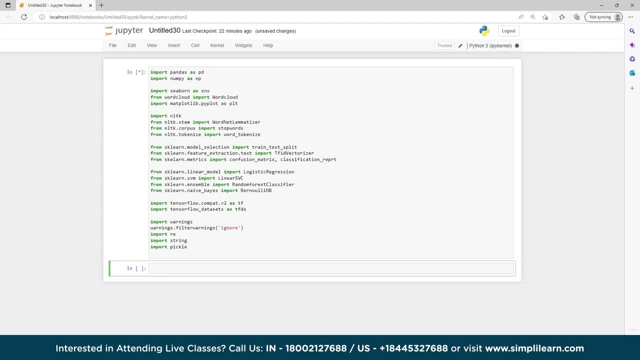 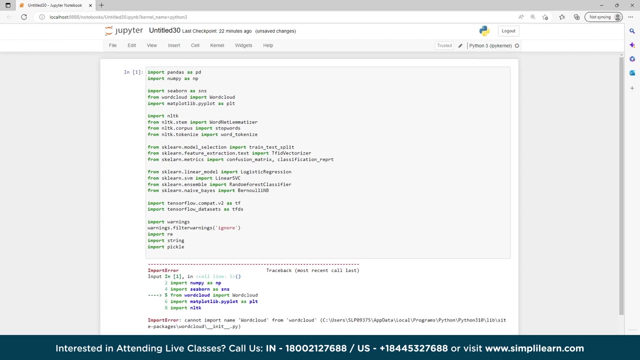 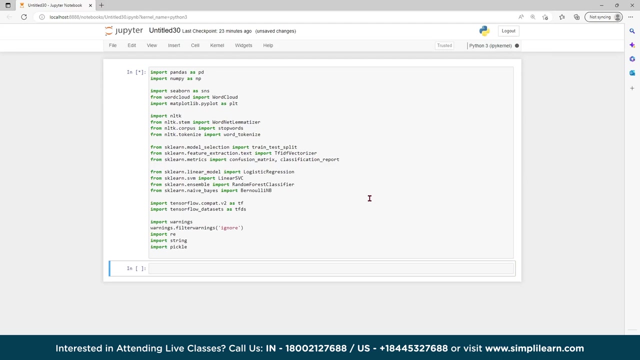 okay, let's run it. let's see how many other. after that, we will load the dataset and we will go through the data visualization. okay, word cloud cannot import name word cloud. okay, see, see, will be capital here, random forest. it's still loading here, let's see. okay, so loading is done, so now let's load the. 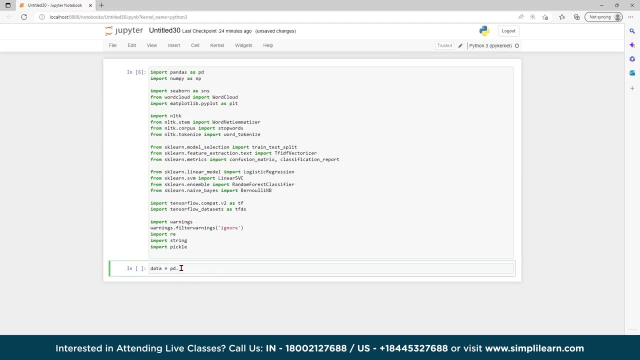 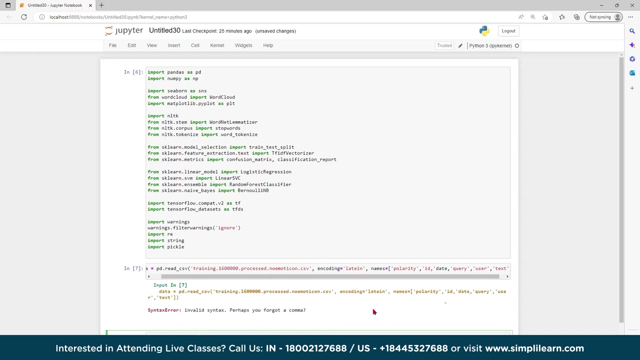 data set. so we'll write: data equals to PD, dot read and let's go. CSV does her name first, you, so you can find the data set. on the description box below. coding goes to Latin first. clarity, you, you, ID, come on date. very you, you, I'll see you forget, come over. 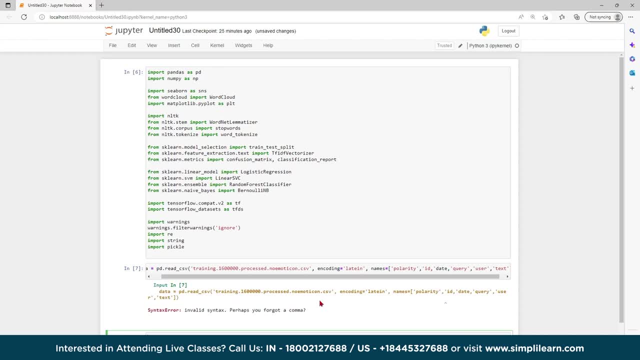 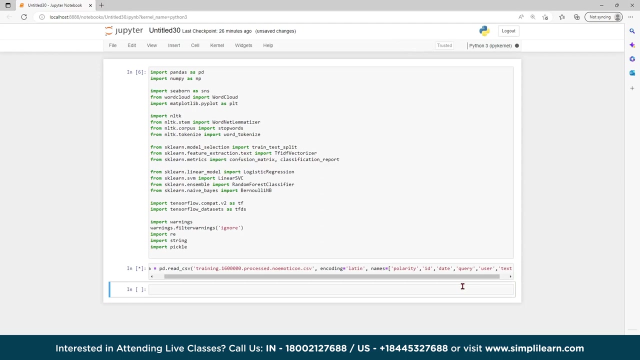 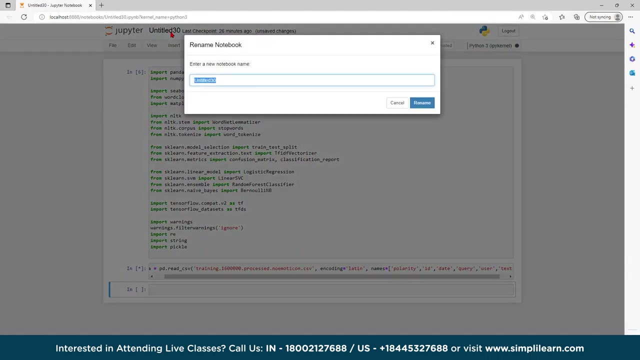 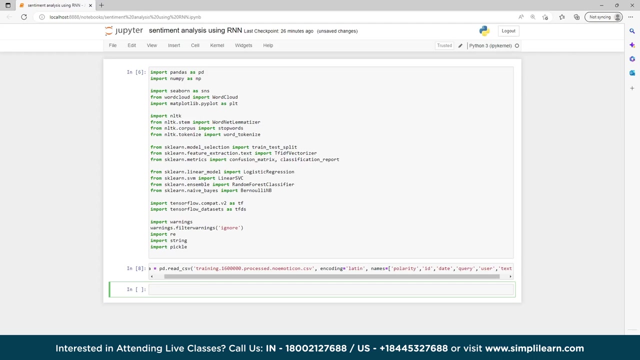 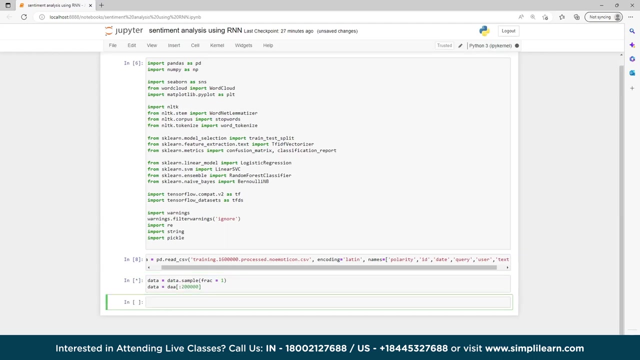 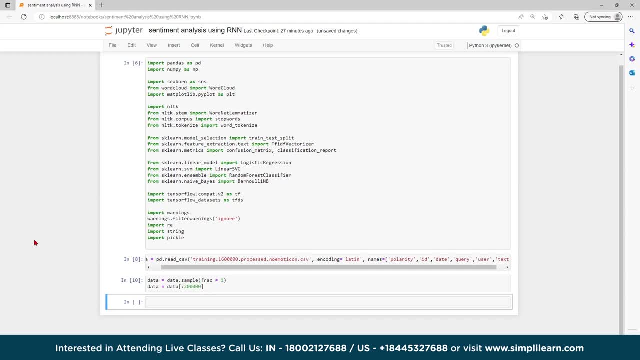 so in this demo, like you will see text processing on Twitter data set and After that we will perform different machine learning algorithm on the data, such as logistic reaction, Random forest classifier, SVC name base to classify positive and negative dudes. After that I will also build RNN- recurrent neural network. 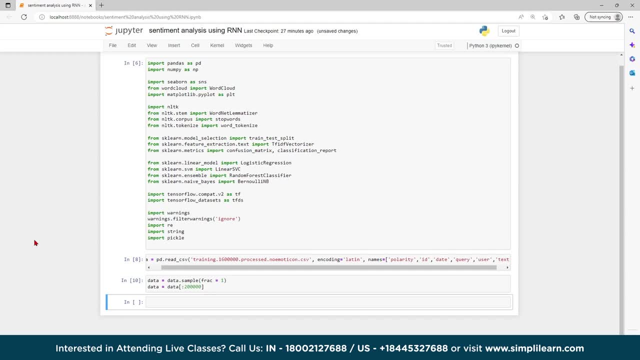 Which is the best fit for such textual sentiment analysis. Okay, since it's a sequential data set which is requirement for the RNN network, So let's dive into. so now We will see the data. data visualization, data set details, target, like the polarity of the tweets. 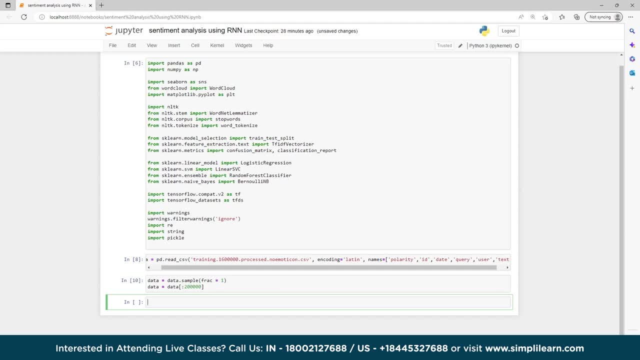 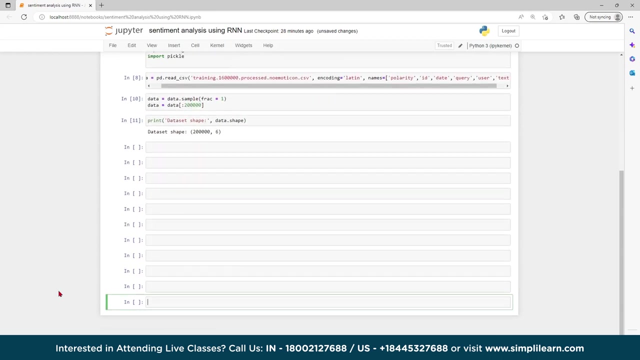 0, negative. Okay, then the date, like date of the tweet and the polarity and the user that what tweeted, then the text: Okay, so I will write print y'all. So here is the data set Set, If You done on my shape. okay, Let me first do like this, ya. 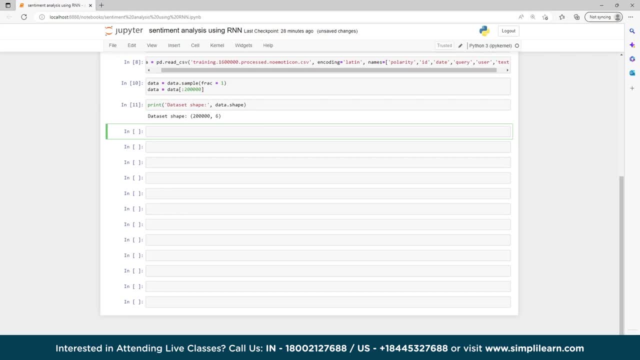 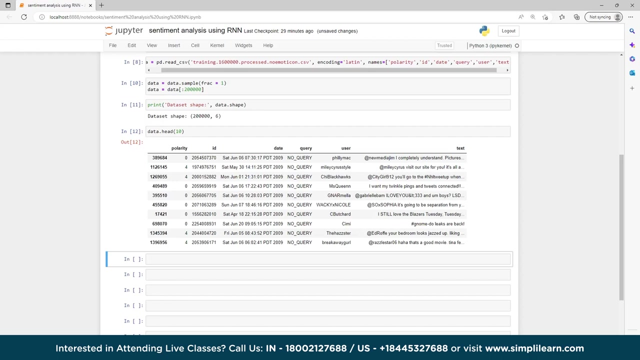 so there are 20, or or you can say two like rows, and six number of columns. okay, so it is a huge data. i will. you can find this data set from the description box below. so here let's see the data and why i use head. head is used for like, for showing. 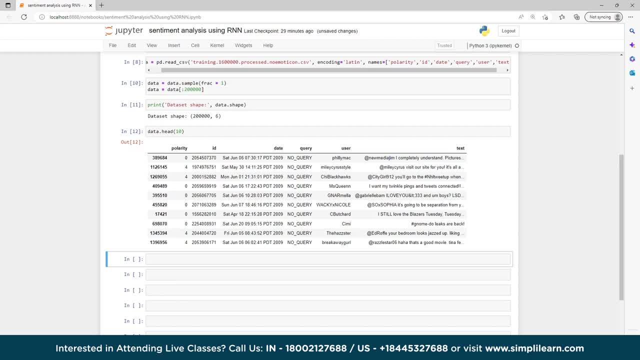 top 10 rows of the data set. if you will use tail instead of head, it will show the last 10 rows of the data set. okay, here polarity 0, 0 means negative and 4 means positive. okay, like you can consider as 0, 1. this is id date, then query, then user, then the text. 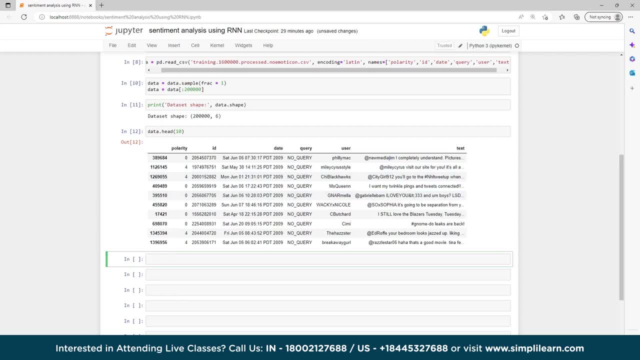 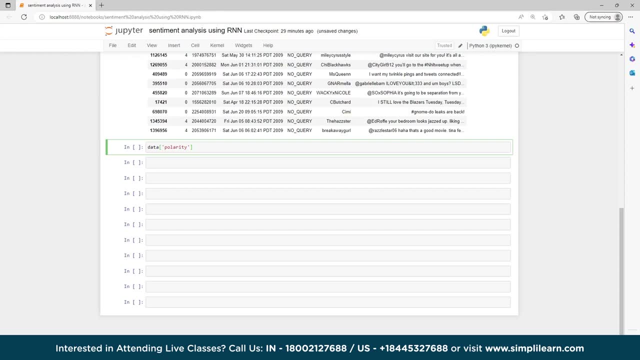 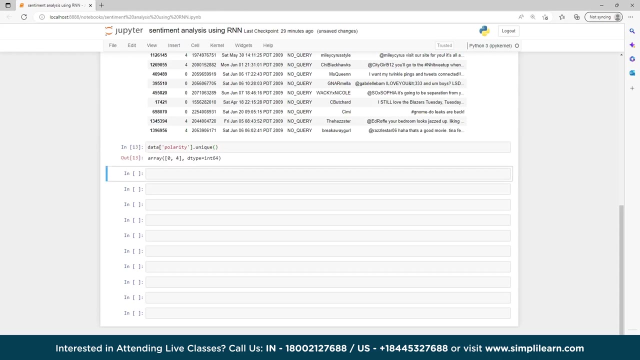 okay, okay, so then i will do. data polarity: okay, these are the 0- 4. okay, uniqueness: 0 means negative and the 4 means positive, replacing the value 4 as one, for the ease of understanding what i said to you. you can consider as zero. 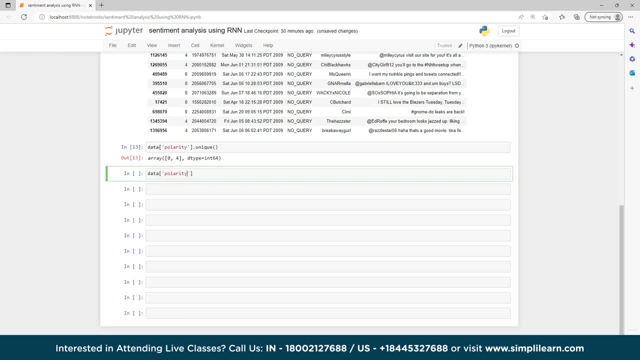 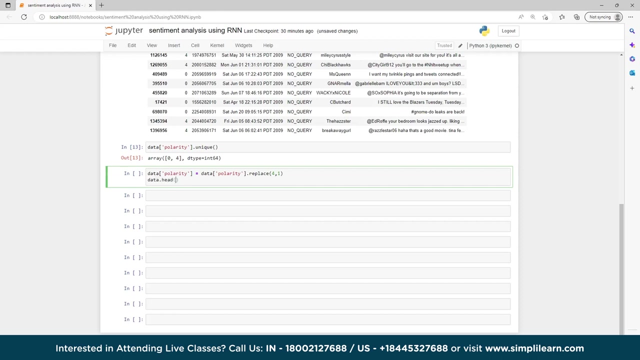 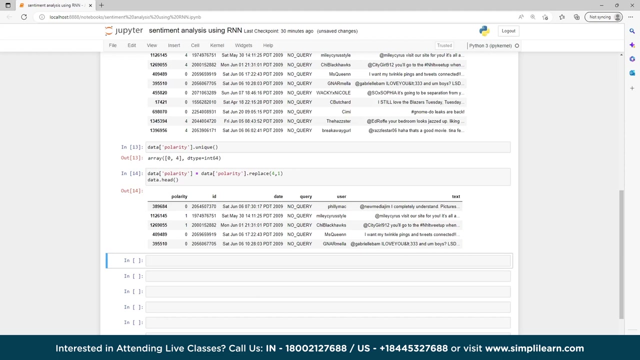 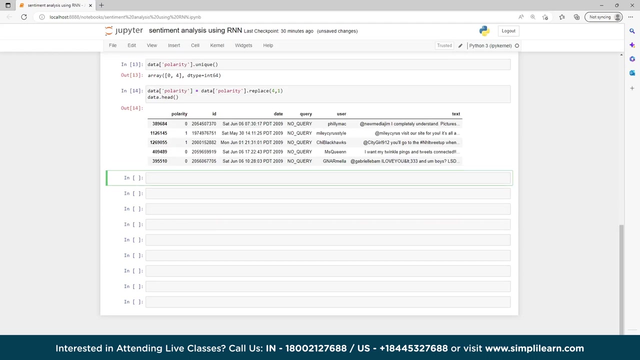 one. so date, data, polarity, data polarity 421 and then data 01010110. ok. so if you will write only head, it will show the top 5 rows only. ok. so now let's use one python function. describe data dot type. so, as you can see here, 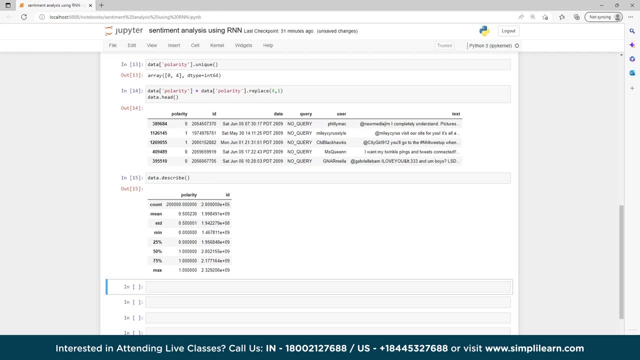 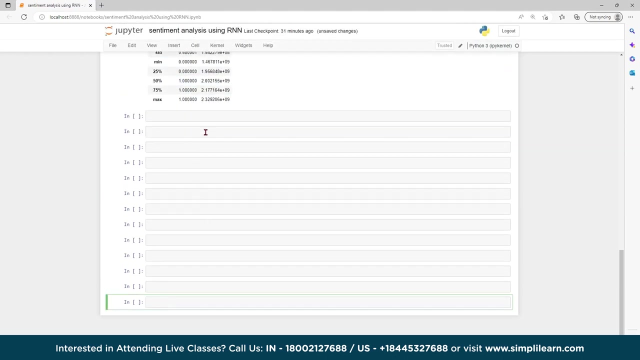 the count is 2 lakh and the mean of the particular row is this and the id is this: standard deviation. minimum value: 25%, 50%, 75% and the maximum: ok. so let's see the number of positive vs negative tagged sentence. ok, so here I will write positives. 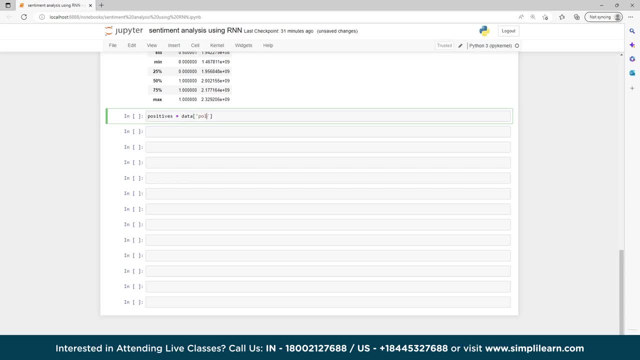 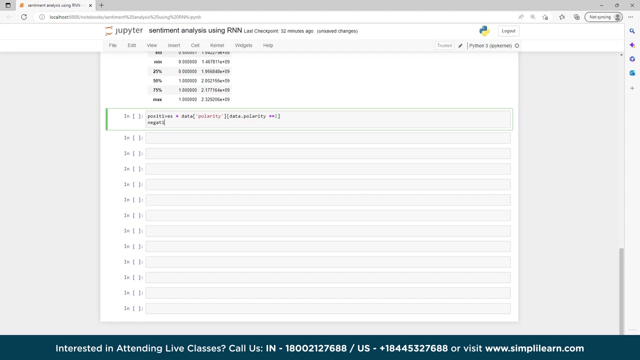 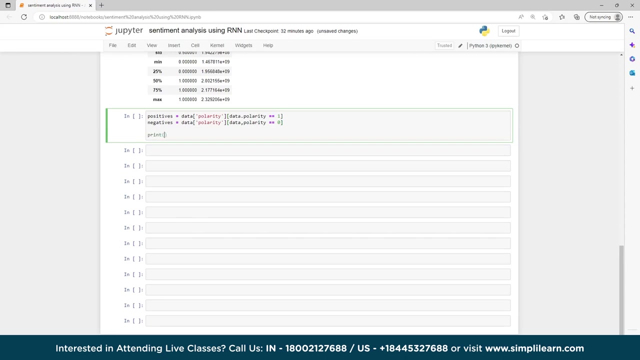 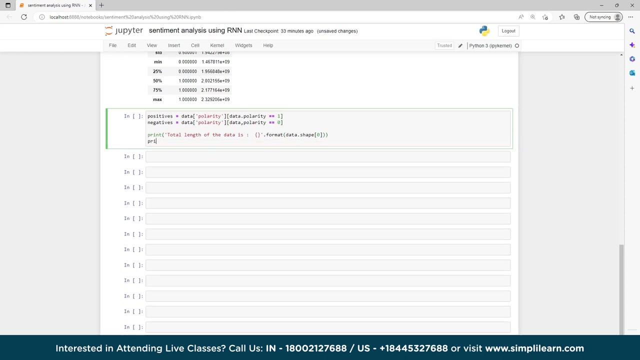 equals to data polarity: data dot polarity equals to 1. then negatives: data polarity: data dot polarity equals to 0. print total length of the data is dot. format: data dot shape: data dot shape. now I will print the total length, the negative and the positives. ok, so number. 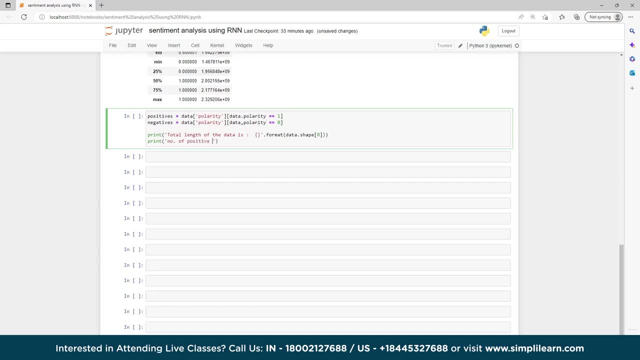 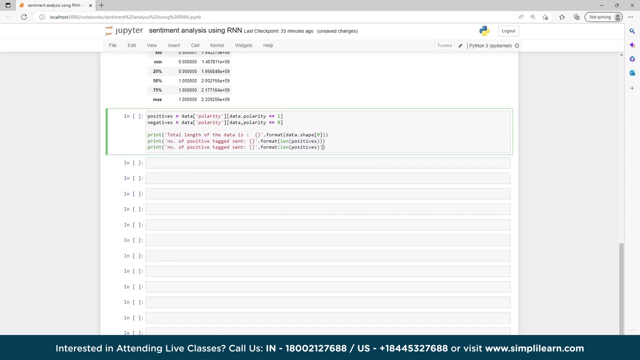 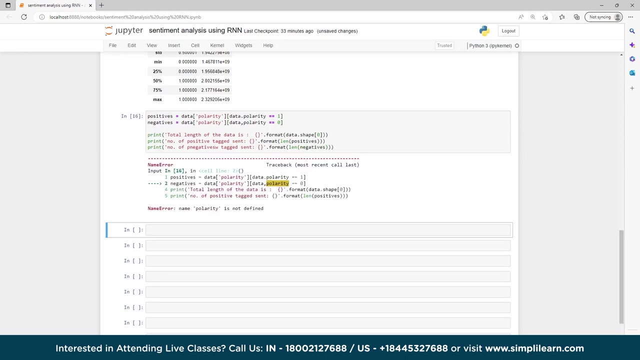 of of I will. let's say this and paste it here, and here I will do the changes for the negatives. now let's see. so here polarity is not defined. so, as you can see, the total length of the data is 2 lakh and the number of positive 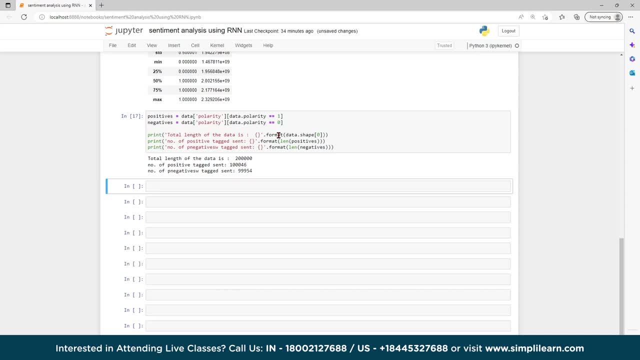 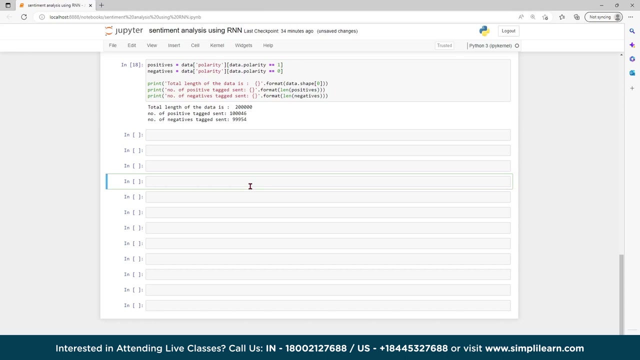 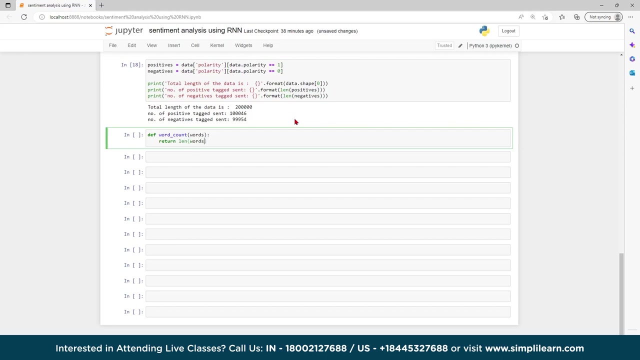 sentences is like 1 lakh 46. number of negatives: okay, spelling is okay. the number of negative text sentences: 99954. okay, so now we have a brief data. so now let's get a word count per of text. so for this I will write, and now let's plot a word count. 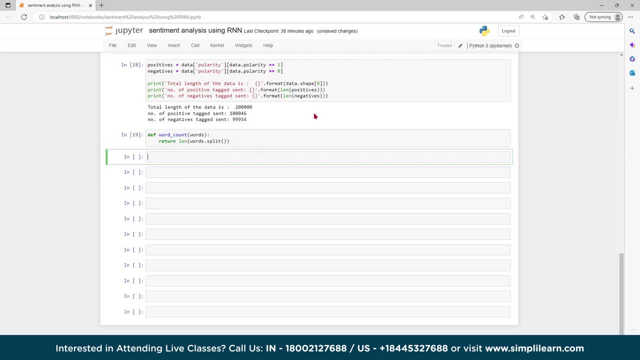 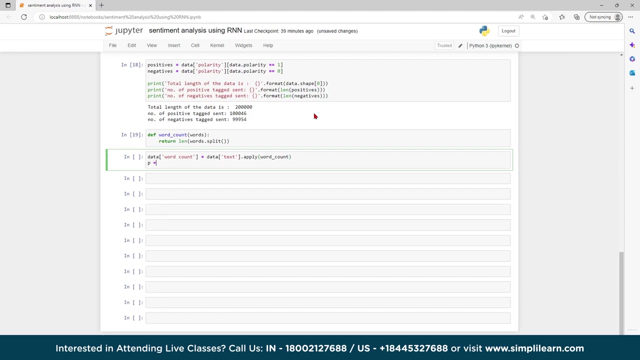 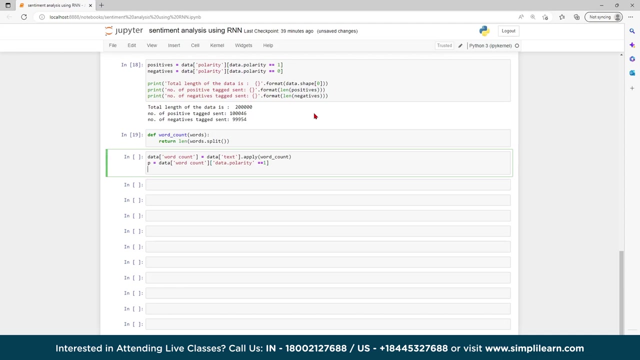 distribution for both positive and negative. so i will create a bar plot. so for that i will write it. word count- data text dot apply word count. okay, then i will write: p- positive equals to data and count: data dot. polarity is equals to one. and let me copy this only: 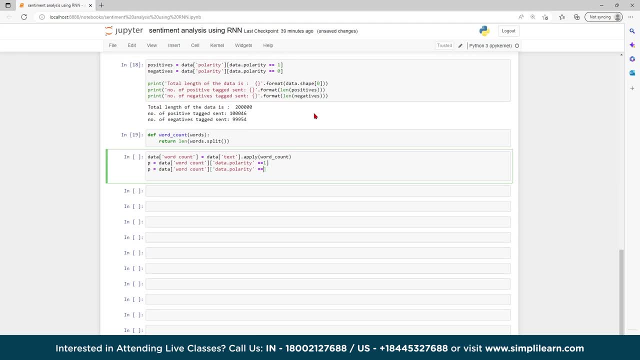 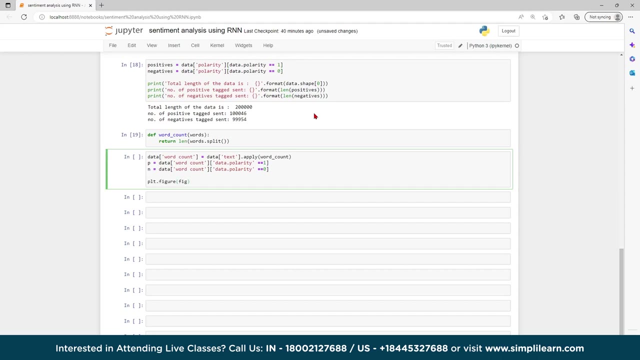 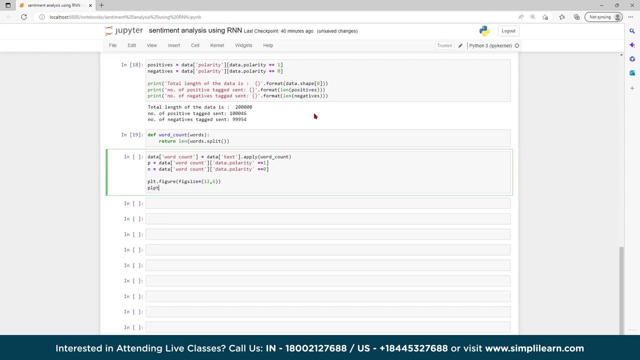 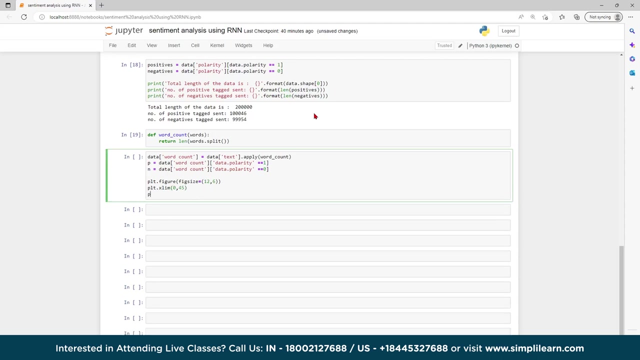 here i will write zero, and okay, then plt dot figure and figure size, question 12 comma 6, and then p l t dot 8 comma 45 and p l t dot x label. word count: one zero and then high, and then well, and then so i will write: 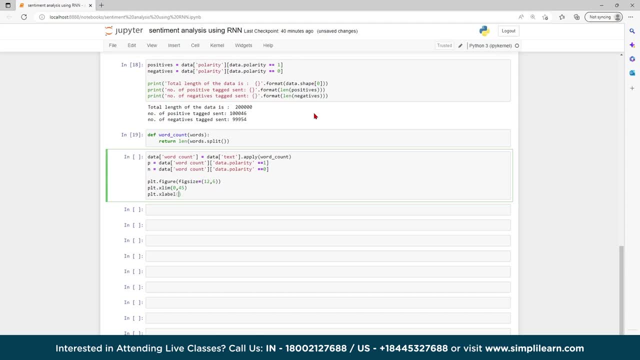 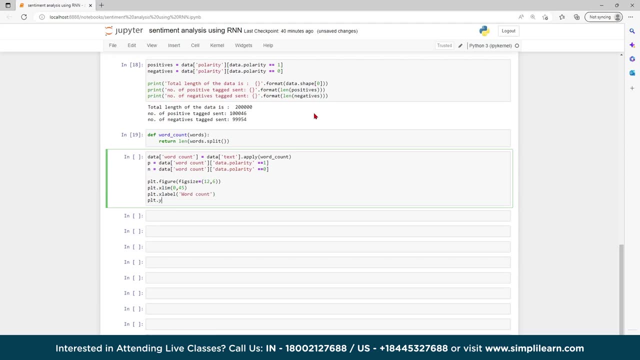 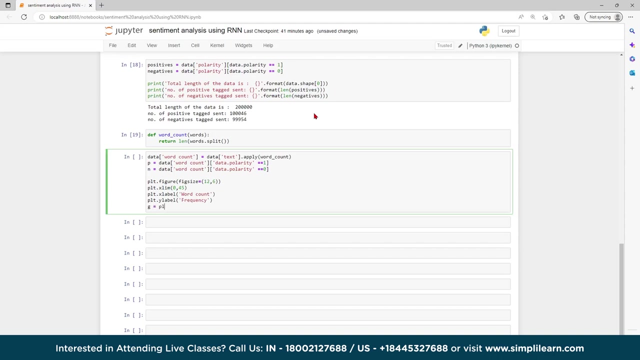 p l t dot. it means number five, two, three. PLT dot Y11 and frequency, and we will write G per se: PLT dot, comma N and color is alpha equals to 0.5, and it is equal to 0.5. and let's make a legend also. 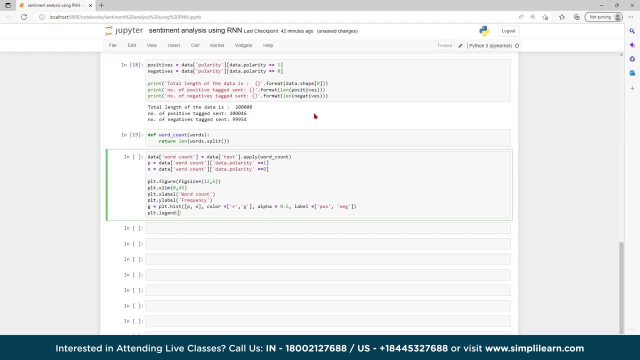 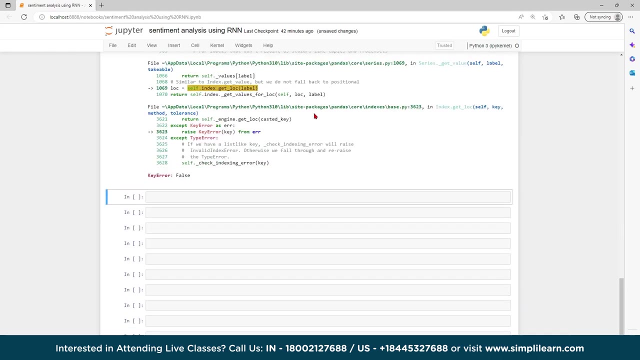 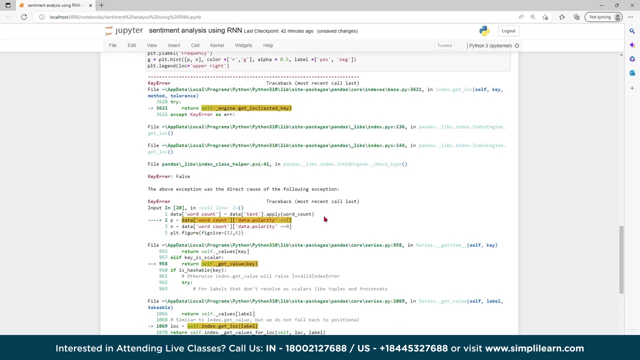 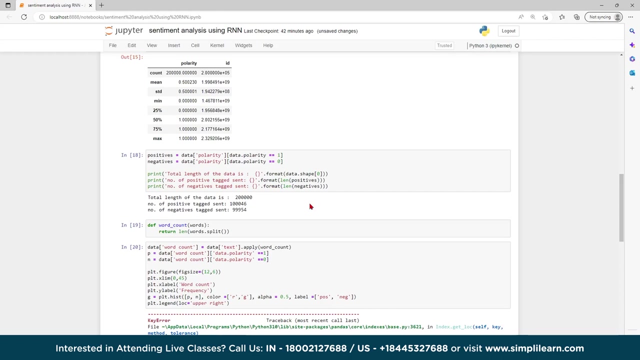 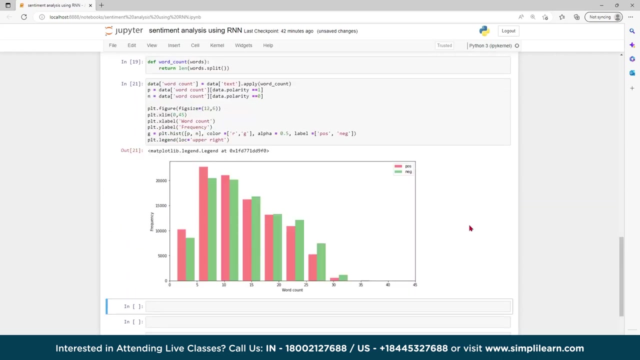 location should be right, false, and data word count product equals to okay, my bad, as you can see, the positive and the negatives. okay. so these are the like word count distribution for both positive and negative. okay, so now let's uh what we can do. we can do the get like, get the common words in. 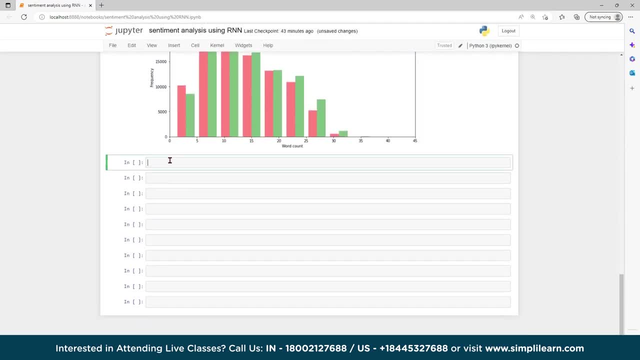 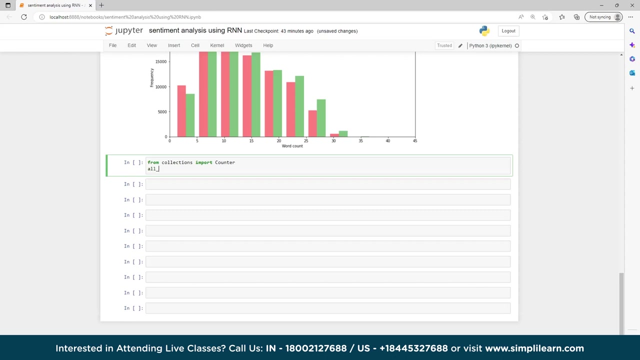 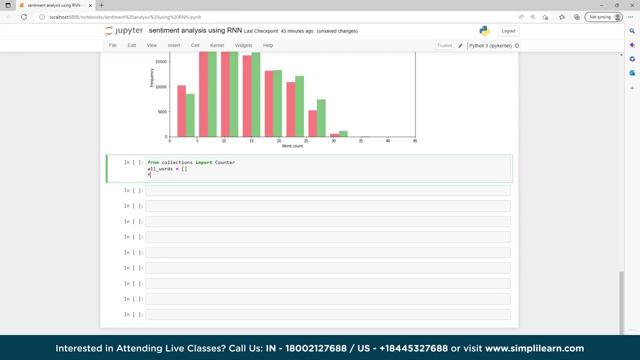 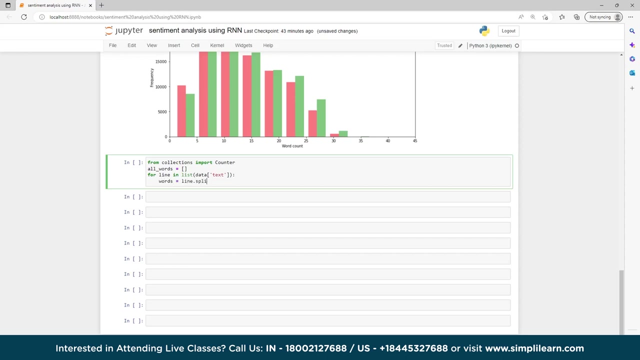 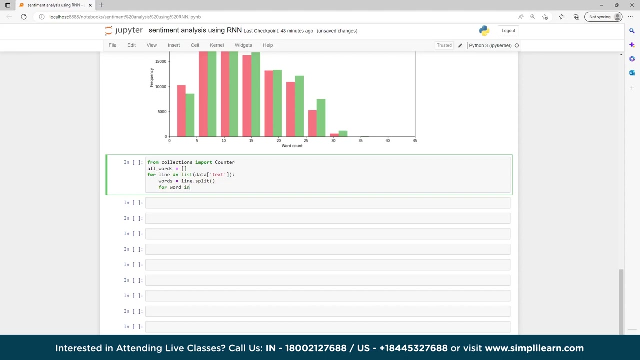 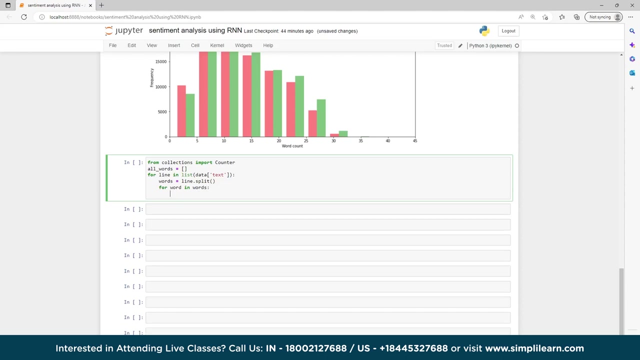 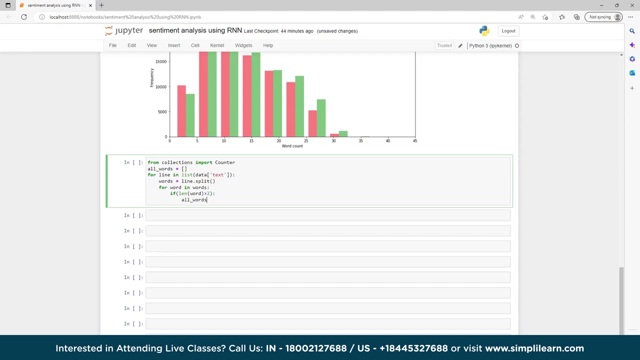 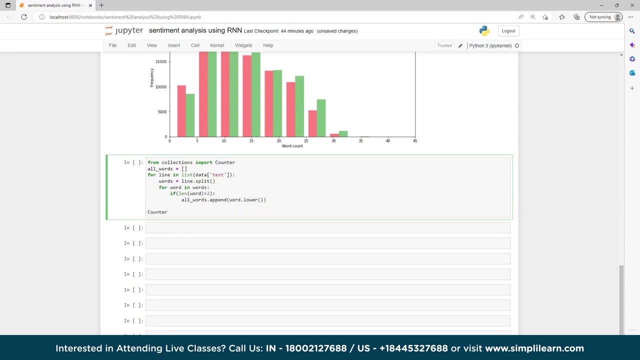 training data set for the training data set. so for that i will do from collections code: counter all words or test data text line dot split for word and words. if length of word is given to line dot, split all dot. here i can write counter all words, not most. 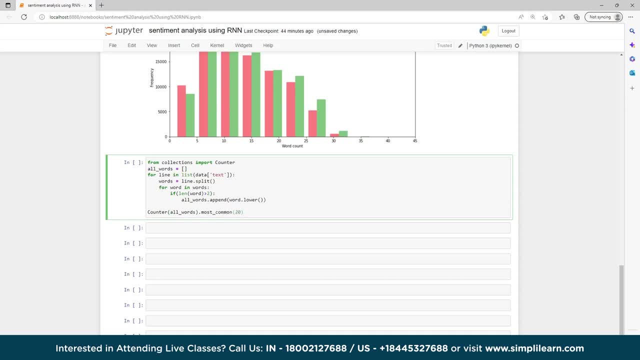 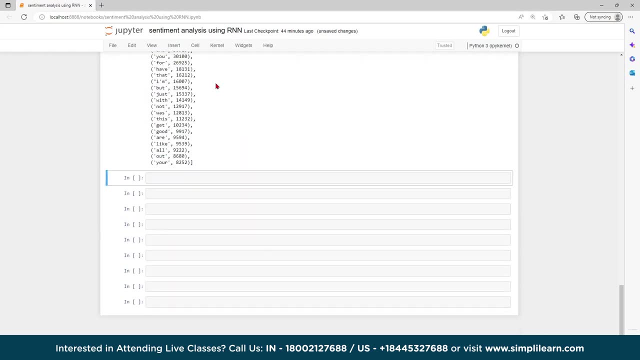 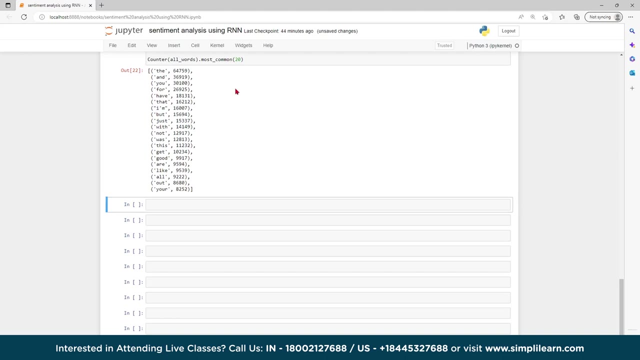 common, then i need 20.. so, as you can see, these are the most common word used, like in every sentence, the, and you for have that i am, but just like this out over all. so these are the most common words. like it used, the is used like 64 000 times and like this: your is used for eight thousand times. 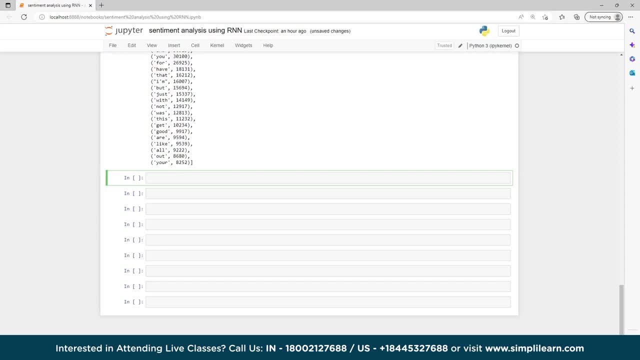 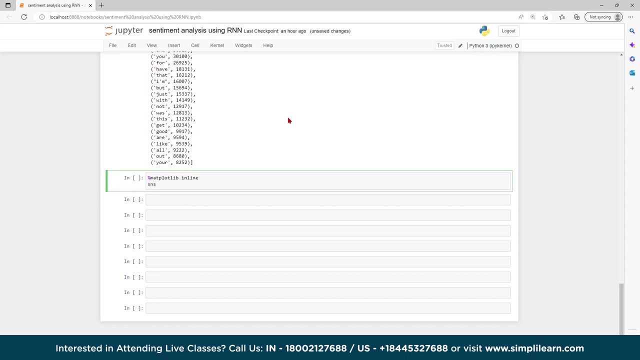 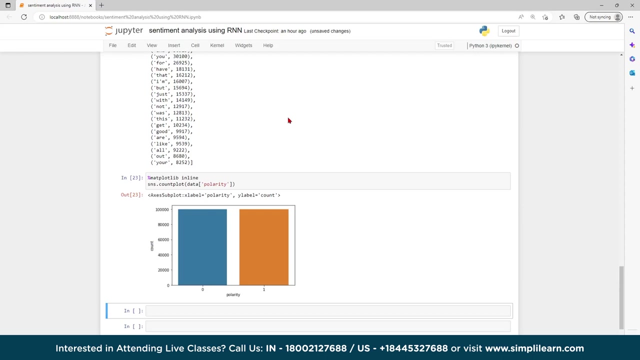 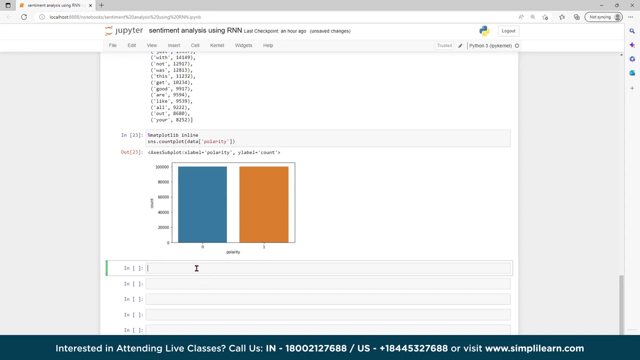 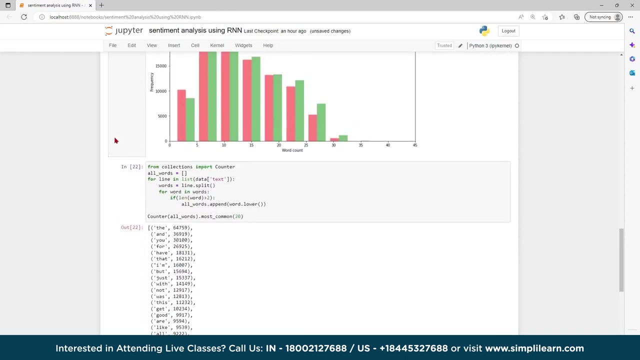 something like that. so now we will do some data data processing. okay, now let's do the data plus pressing and SNS dot count plot data polarity. yeah, these are the negatives and it's positives. there are the slight change. I guess that is why it's not looking so much of. 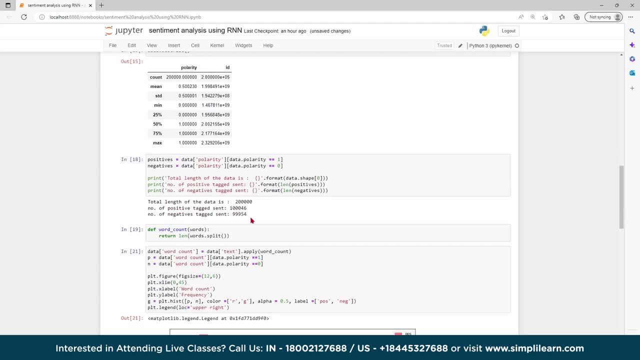 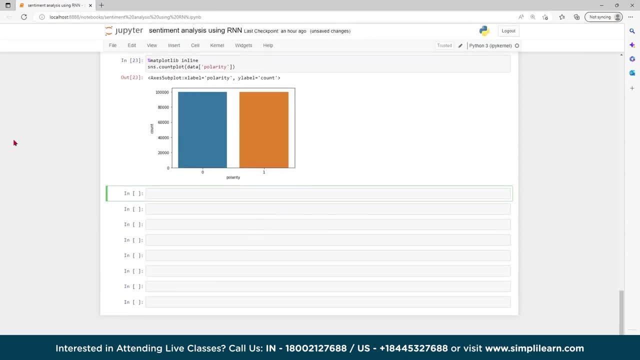 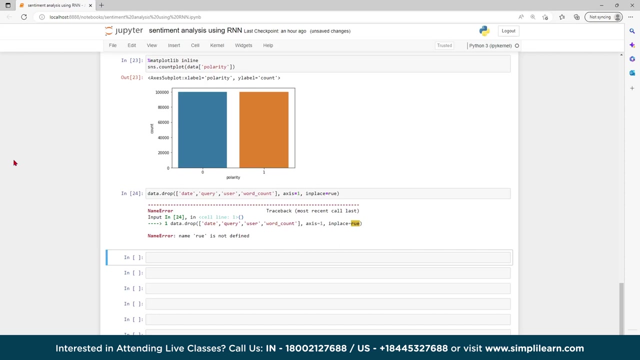 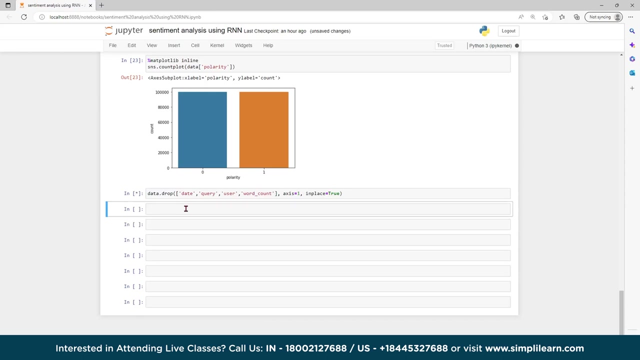 different, like there's a slight 46 different, so that is why it's looking almost same. okay, so now removing the unnecessary columns like query, user, word count, data dot. draw it ready. and what count? this is equals to one comma place question. okay, a true, so here I will write data. 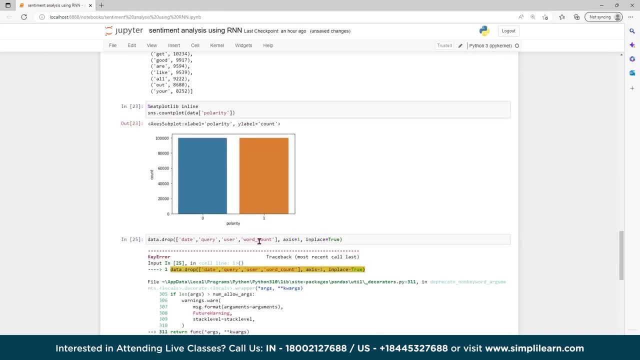 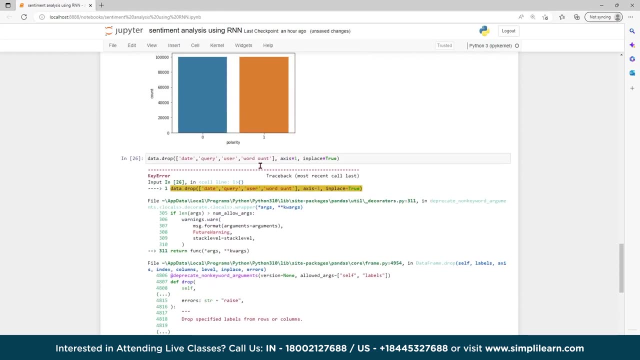 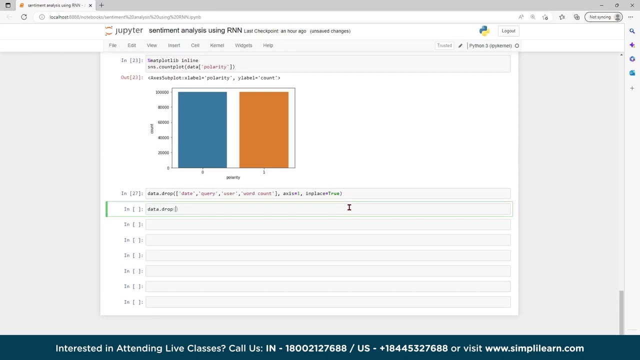 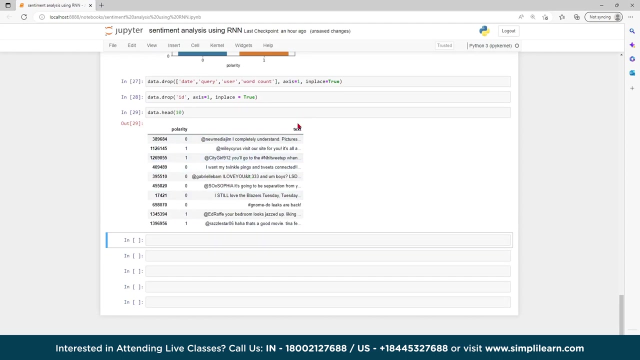 work on this. no, okay, my bad, here I will write data dot drop ID. come on, so one you, you, you To the data. put data dot, add the data. see, we have only at the two the polarity and text. okay, oh, Oh, now let's see the null values. 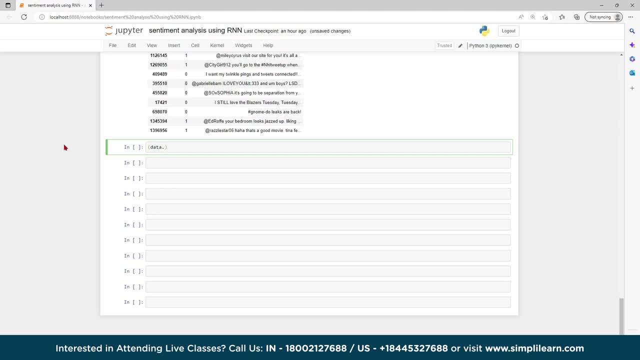 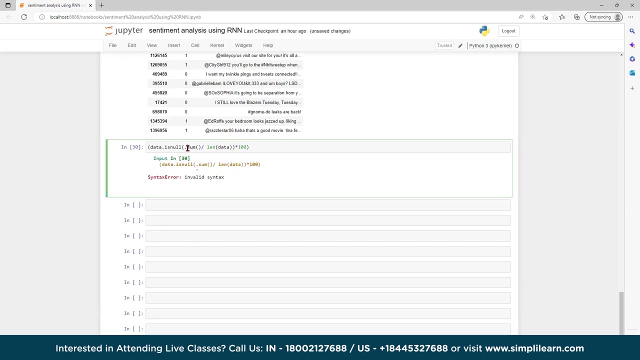 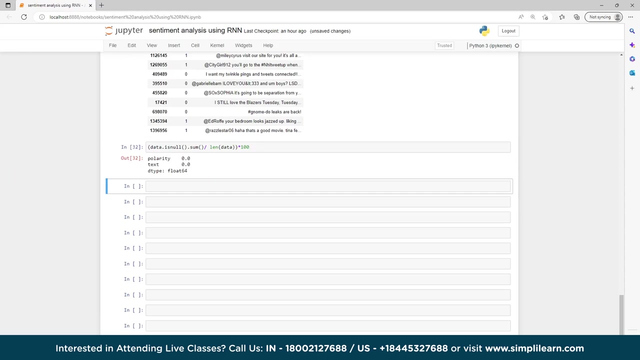 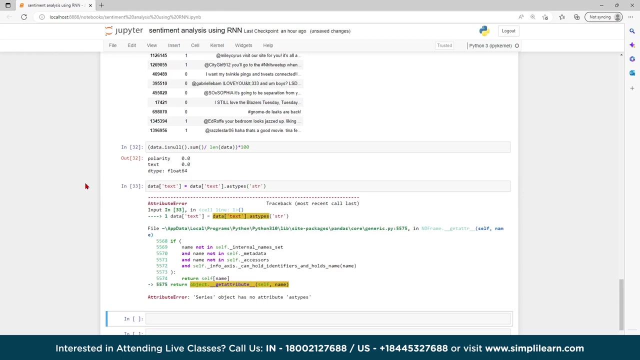 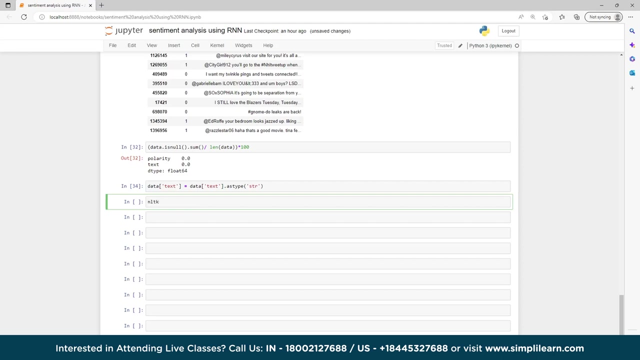 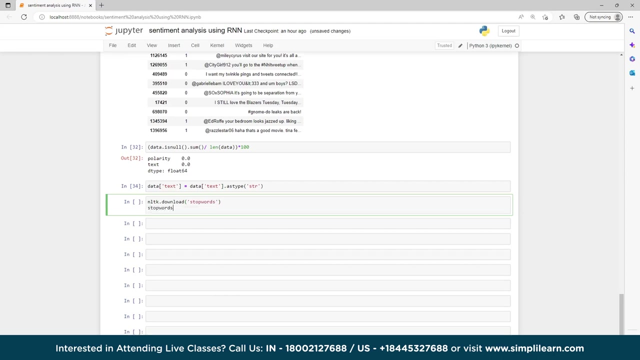 data dot data event. ok, so there is no null values. so now converting pandas object to a string type. for that we have to write text pursuit, data text type: tr object as types. yeah, so now download the stop words: nltk. download words, words, set words. it's in English. 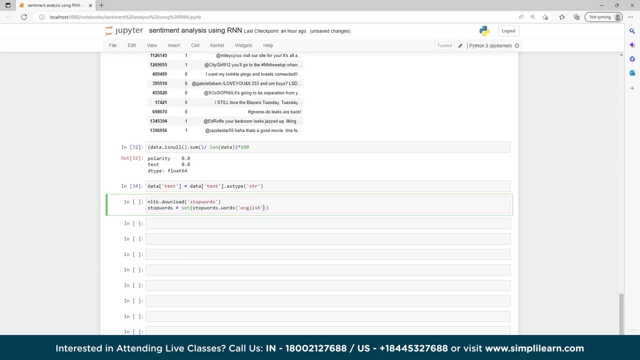 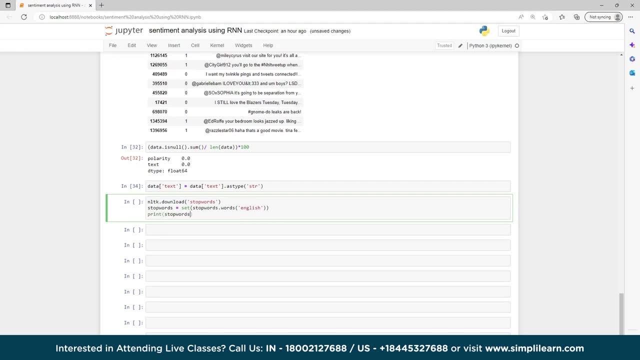 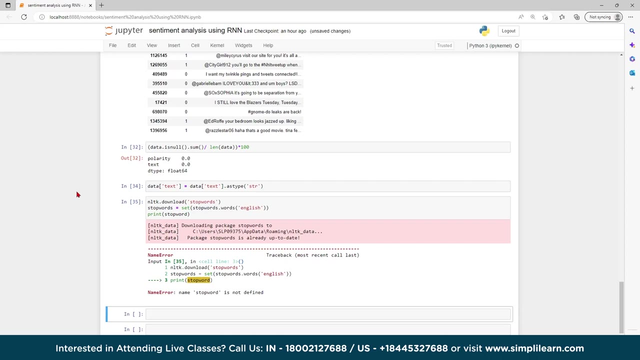 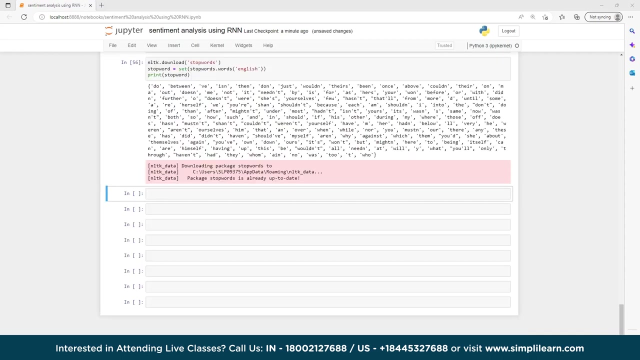 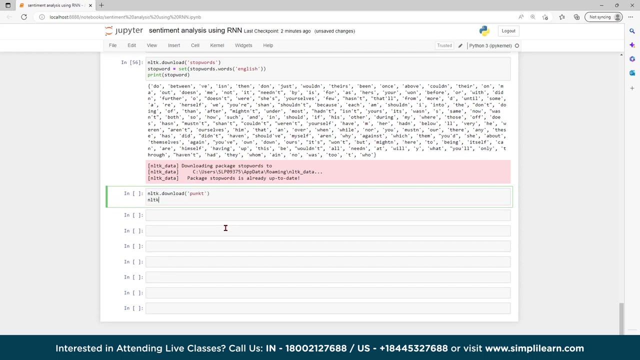 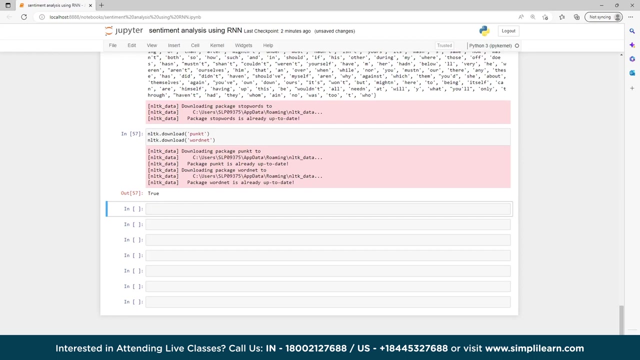 print stop words. this, these are some, you know stop words. so moving forward, let's download nltkdownload. see okay, so the pre-processing steps taken are like lower-casting: each text is converted to lowercase, then remover of URLs will do. this means okay links starting with StpSttp or stps. 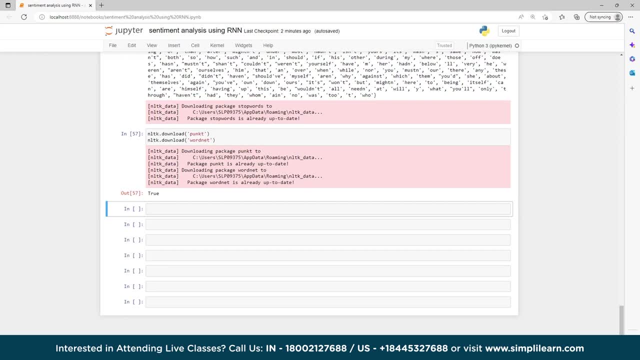 or ww are replaced by remove usernames, shorts words, removing stop words like lemmatization, is the process we'll do of for the converting a word to its base. okay, so for that what i will do, we'll just copy the whole code for you. we'll explain you one by one what i've done. okay, so this is a course for the url. 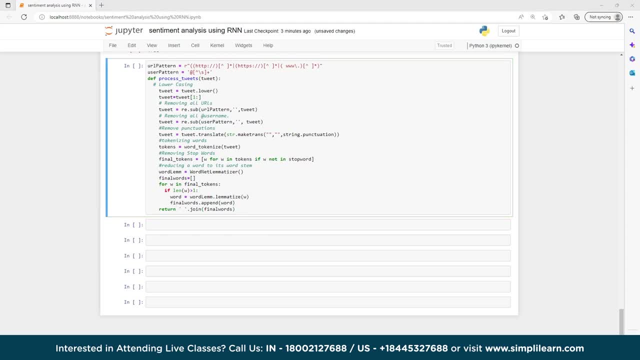 pattern for removing all the www, https and http type of thing and removing them, and i have used pattern for the lower casting: removing all the url- okay, then. removing all the user names, like at the red, and removing punctuations and stop words: okay, like this. so now what we have to do: data. 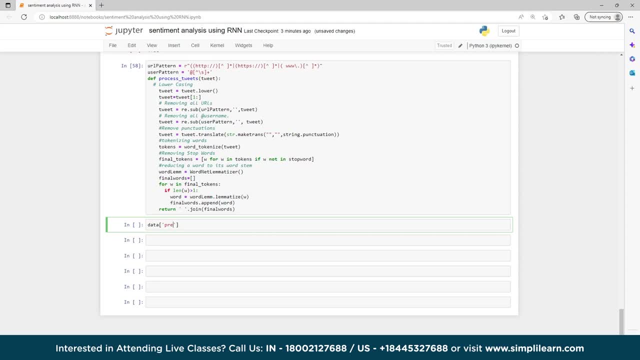 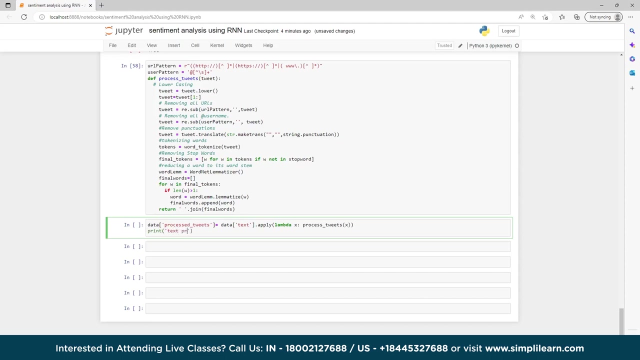 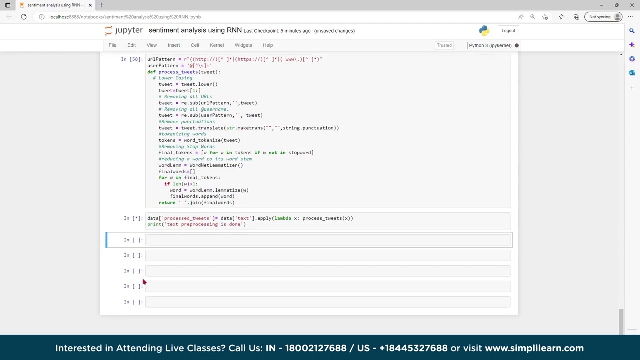 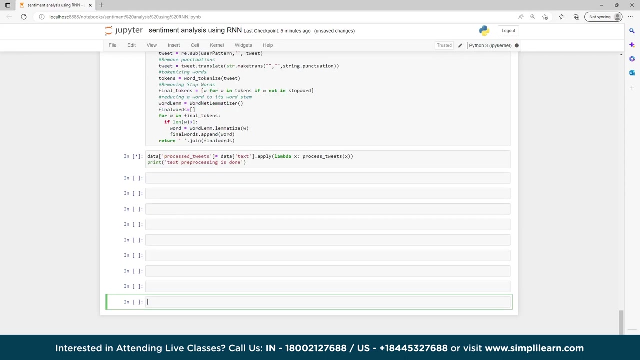 C, the processed tweets, then data text. But apply lambda x, processed, then tweets. okay, Then print text deprocessing. so it is taking time And it will be completed. it will return here. text preprocessing is done, okay. 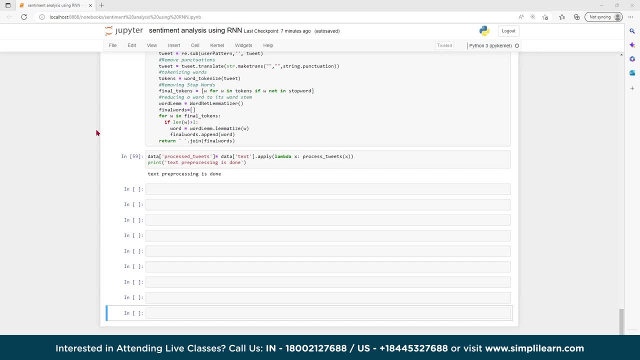 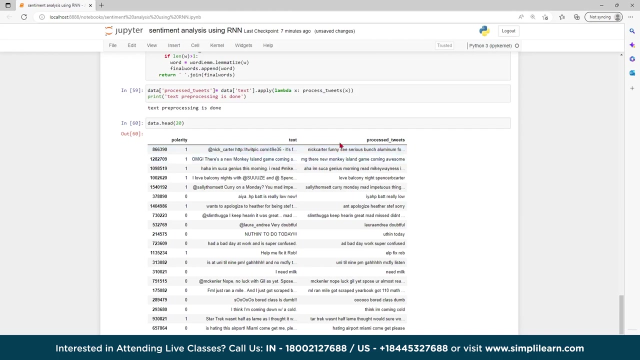 As you can see, the text preprocessing is done. So now let's check dataad. As you can see, the at the rate and this slices are gone. okay, So now the text is preprocessed. So now what we will do. we will analyze the data. 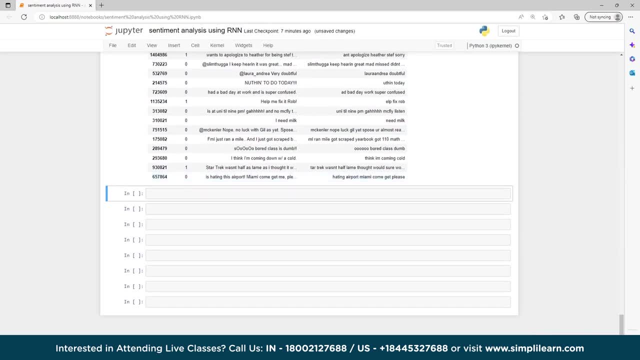 So now we are going to analyze the preprocessed data to get an understanding of it. We will plot word clouds for positive and negative tweets from our data set and see which one occurs the most. okay, First we will Create for the negative words or negative tweets you can say: 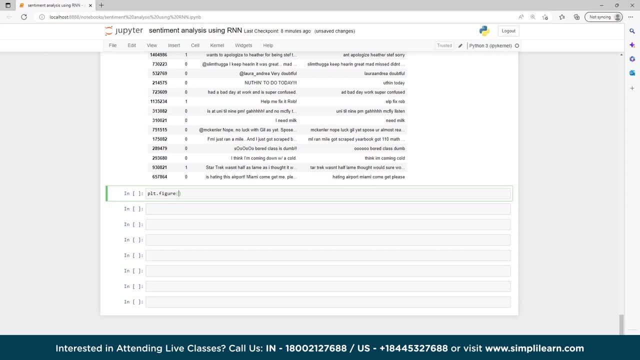 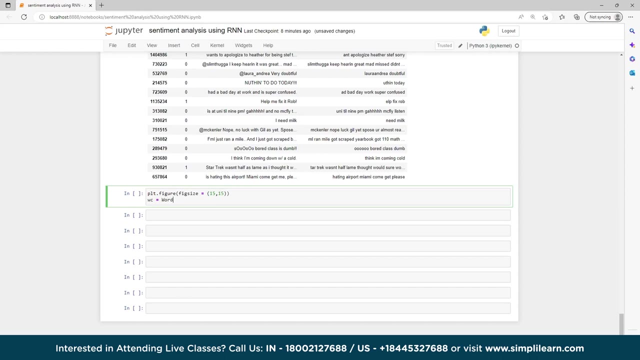 So I will add pltfigure, then figure size: 15 comma 15,. okay, Then word cloud: Person, word cloud, Next words Person, Person. 2000 comma Height equals to 1600 comma Height equals to 800.. 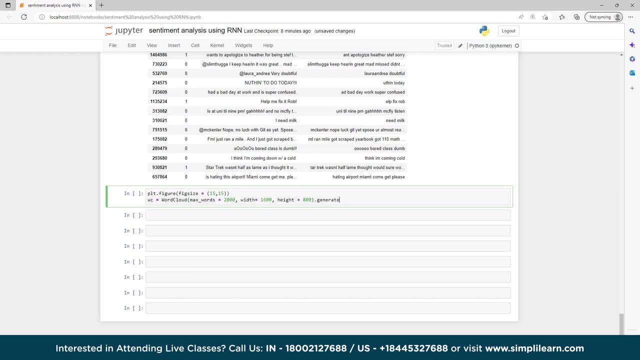 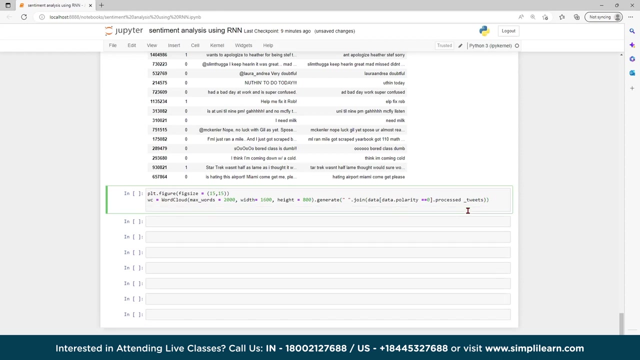 Rate. Join the datapolarity. Height equals to 600 comma. Height equals to 800.. Height equals to 800.. I will write here: polarity: Okay, equals equals to zero. Then processed tweets: Okay. okay, then here i have to write: plt dot show. 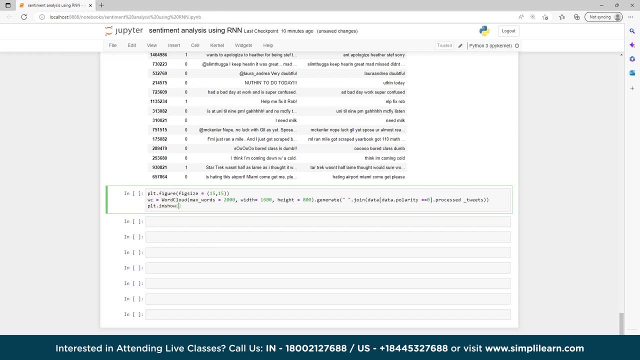 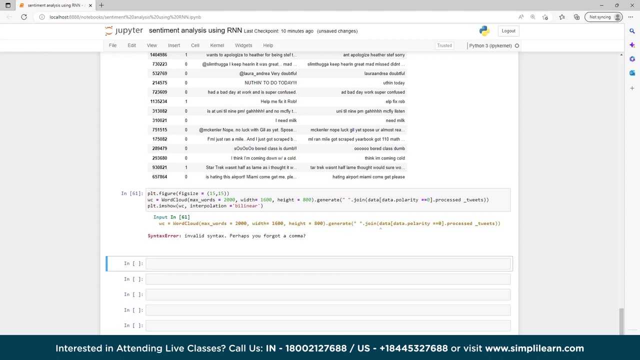 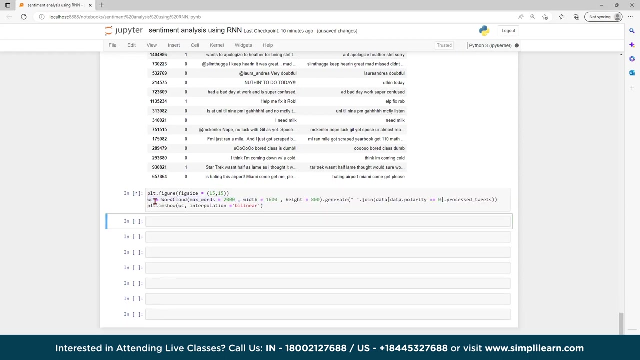 let me show wc interpolation. let's do a linear. if perhaps you forget the comma of here, so 2000, then comma width: dot generate. okay, what i can do, let me run now. let's see. hope this time it will work. okay, it's still loading, so 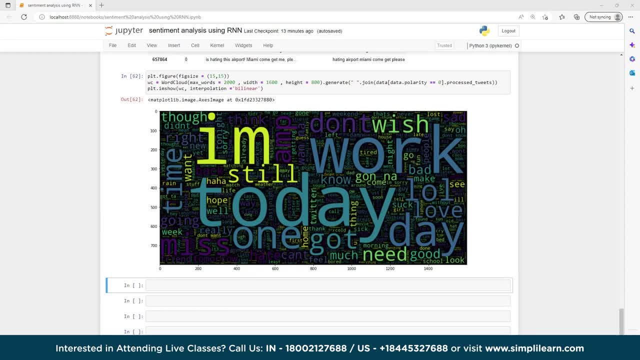 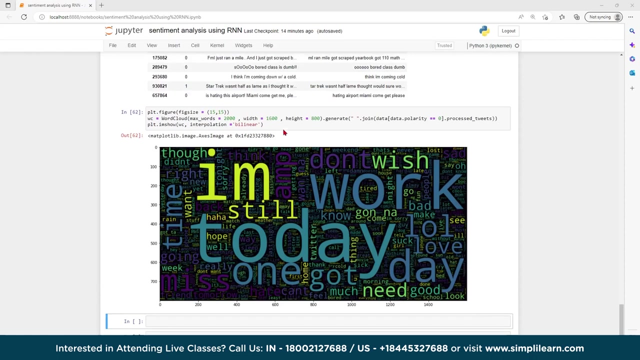 as you can see, this is: it's okay, like today i am and work, don't wish they need my. these are the most negative tweets. okay, words from negative tweets. you can say, right, so let's see the positive tweets. okay, so the thing will be the same. let me copy. 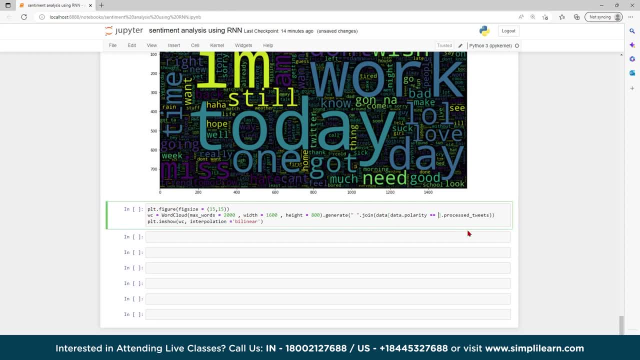 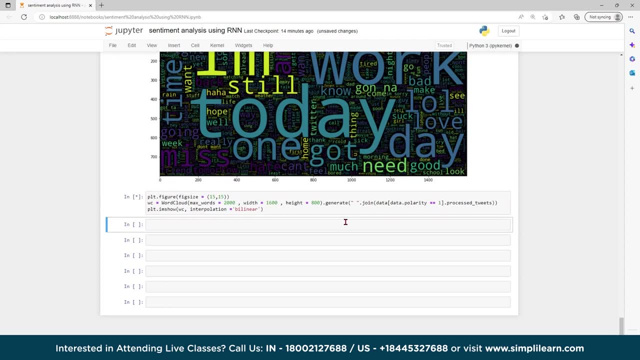 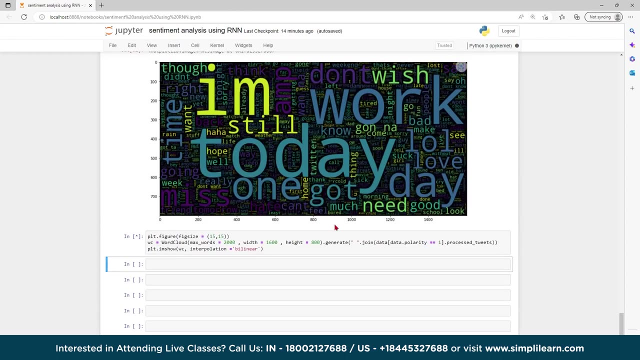 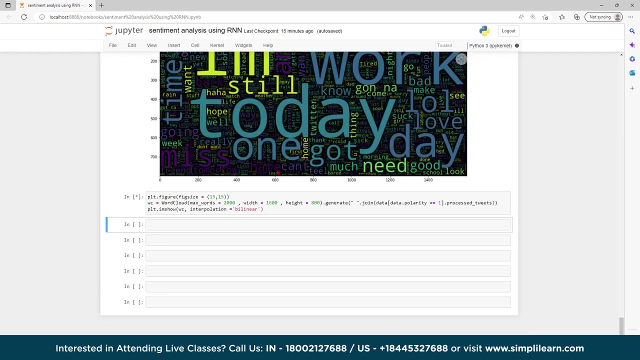 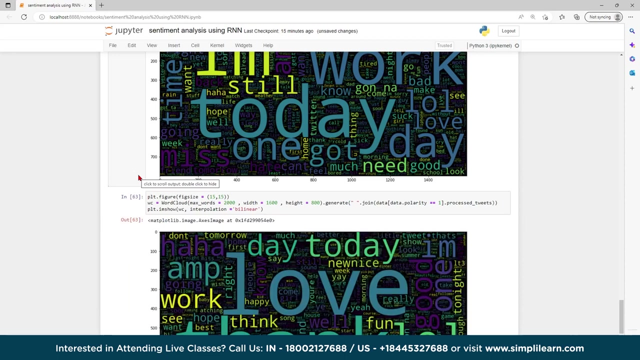 paste it here. so for this i will do one. it will take a little bit of time. it will take little bit of time loading. as you can see, hate can't. okay, sorry, these are the negative words. okay, still loading, so let's wait for a few seconds. 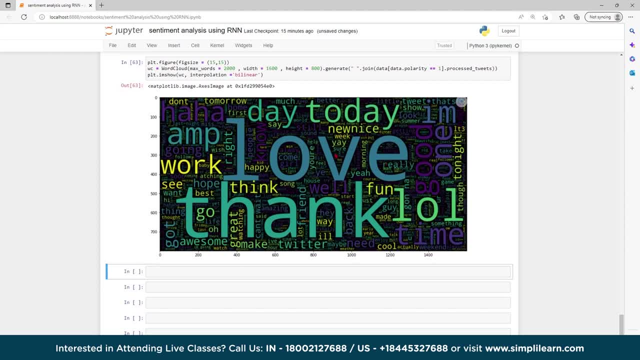 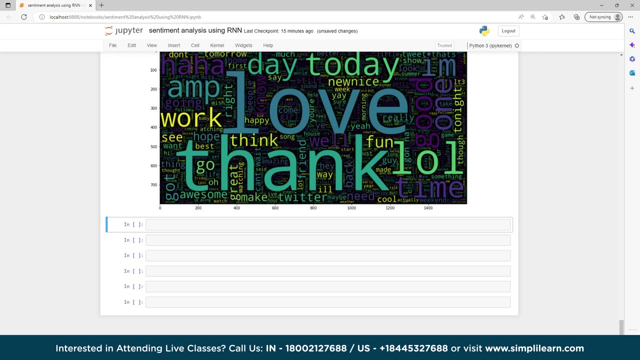 okay, part 2: positive words like love, okay, good, lol and awesome, something like that. okay, so these are some positive words. so now let's do the vectorization and splitting the data, like storing into input variable process to its to x and output variable polarity to y. okay, we'll do that. 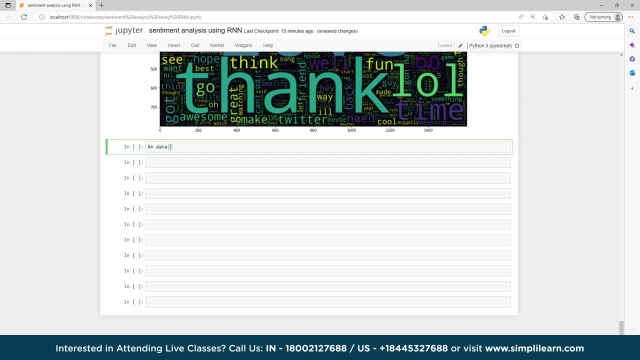 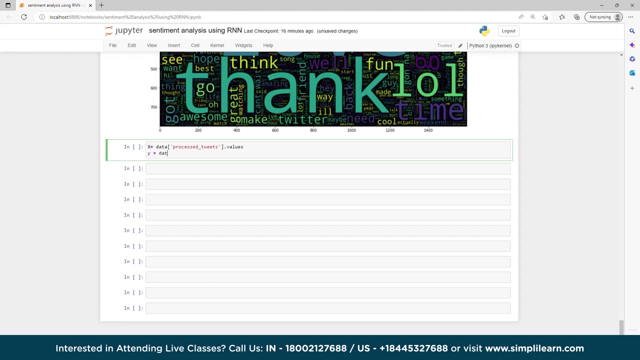 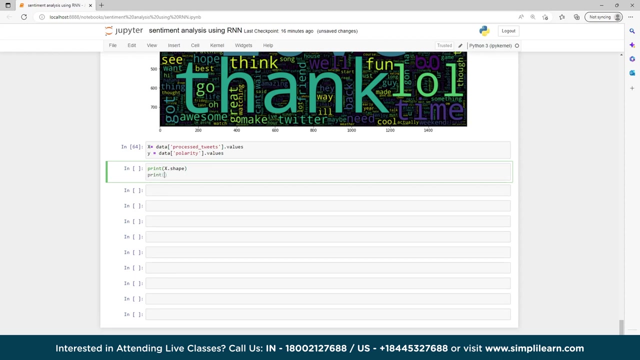 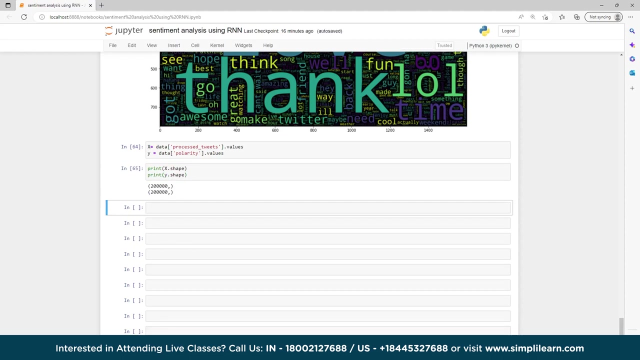 so x equals to data processed tweets values and y equals to data parity dot values. okay, now I will write: print this dot shape. print y dot shape. okay, cool. so now what we will do. we will convert text to word frequency vector. okay, tf to idf. so this is an acronym that stand for term. 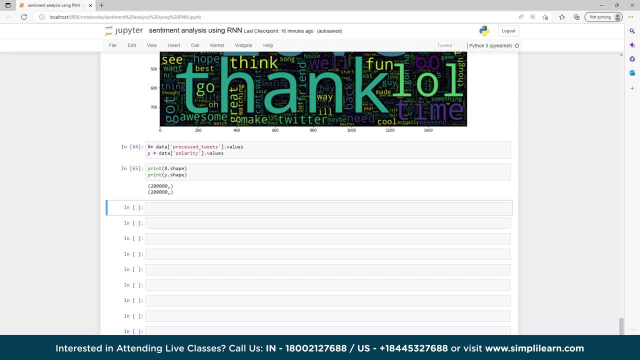 frequency to inverse document frequency, which are the components of the resulting scores assigned to each word. okay, so term frequency: this summarizes how, upon a given and word appears within a document. and inverse document frequency: this downscales word that appear a lot across documents. okay, so now here we will convert a collection of raw documents, so a matrix of tf, to idf features. 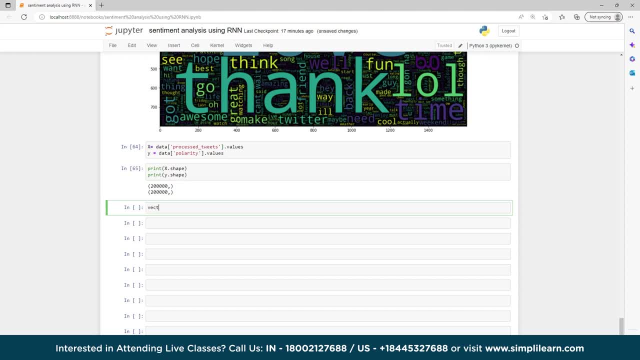 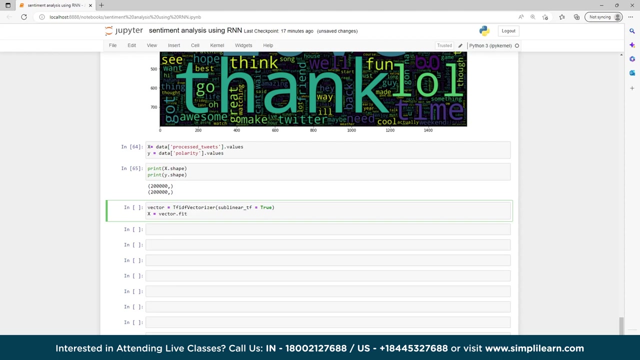 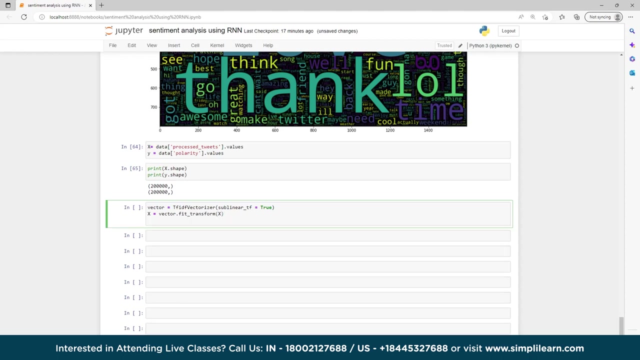 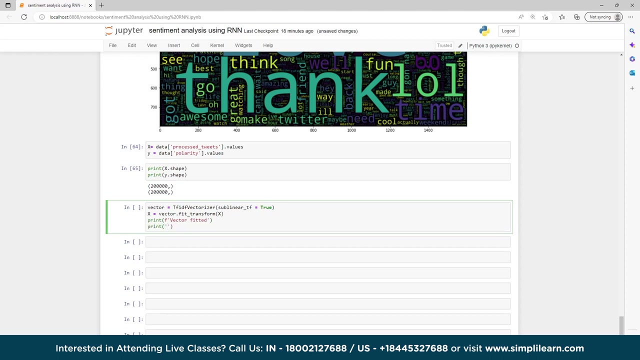 okay, then I will write: enter kazuti fidf advertiser and sublinear in the and sub linear engine this two: yes, this equals to vector dot bit transform and print fixed change this. okay, now we will do the next point. x equals to the did game and number on: 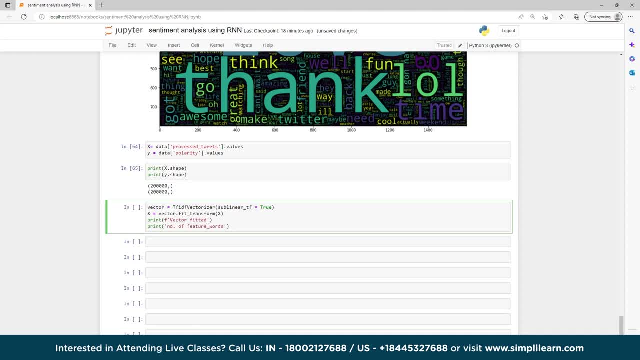 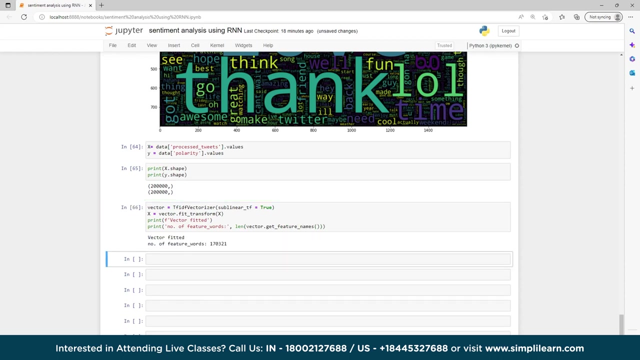 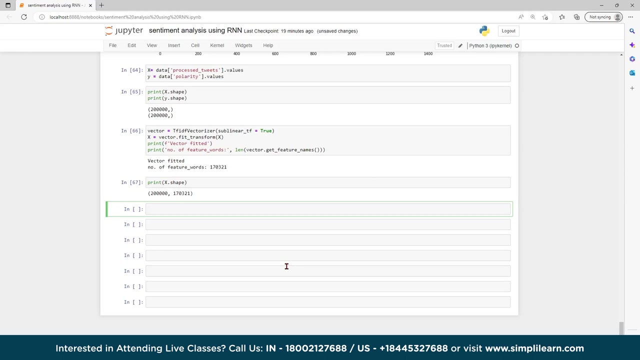 feature, among them actor. yet, yeah, number of feature words are like 170321. ok, now we will do like on let's and ship. yeah, so now we will do the split- split to train and test. so the pre-processed data is divided into two sets of data: training data and the testing. 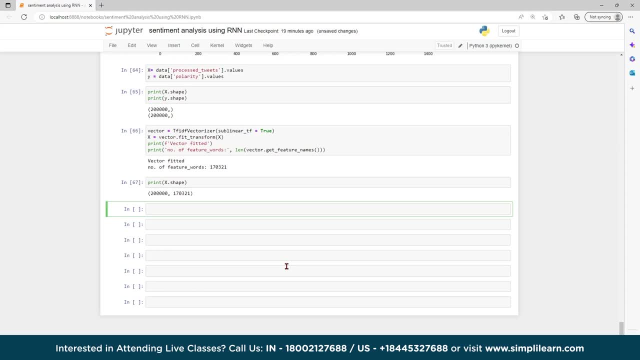 data. so data set upon which the model would be trained on contains 80% data. the test data is that data set upon which model would be tested again contains 20% of data. so for that I will write text: train test, train. come on and test. 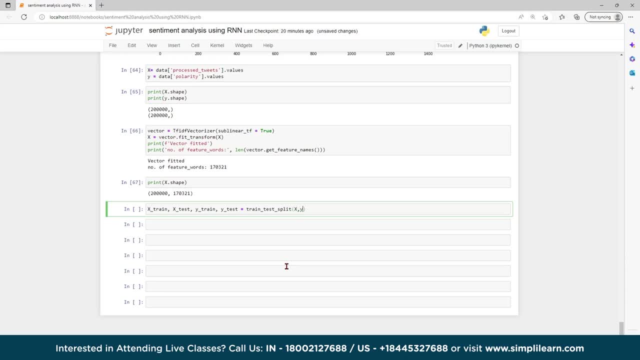 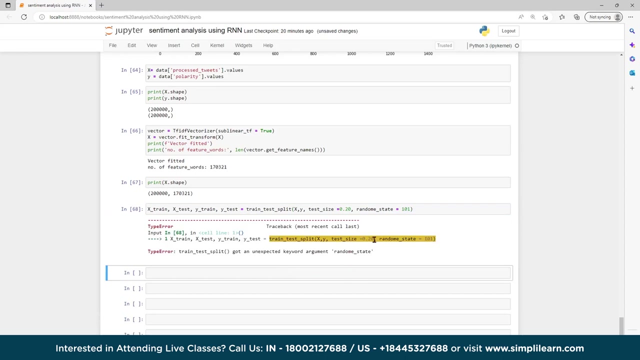 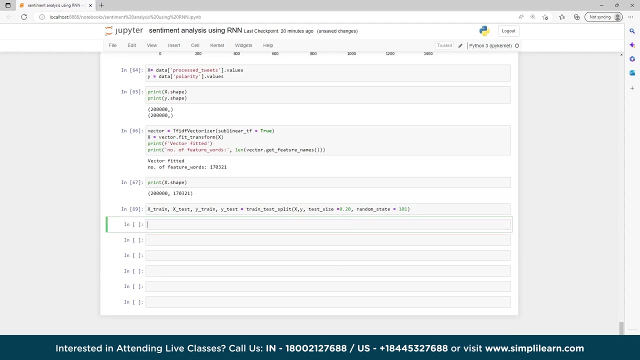 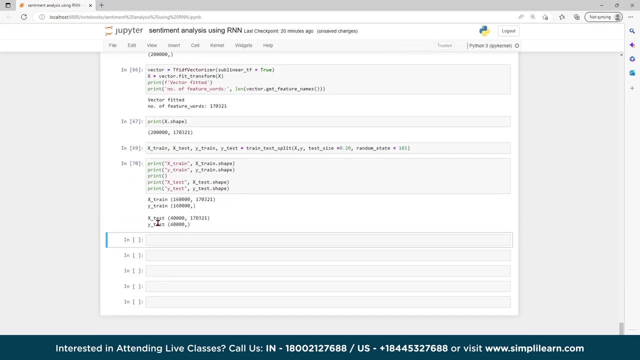 speed and update with some text. two, and- and i've got a file here, so that's, that's should be knows, okay. so now let's do the model building. okay, model evaluating functions. so now let's make a model. okay, and first I will do, I will write, and then I will explain you the whole, okay. so here what I did it. 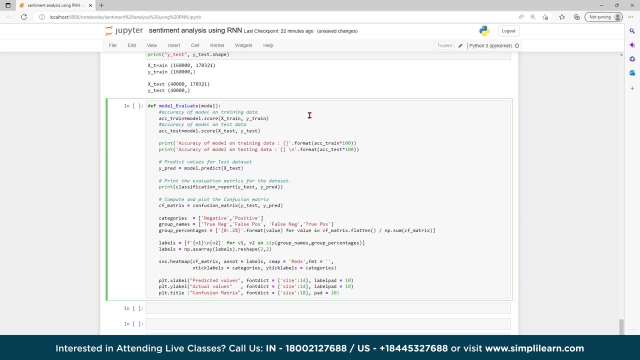 this will tell you the accuracy of the model of training data and the testing data. okay, then we will predict the values for test data set and the evaluation for the data set. then we will compute and plot the confusion matrix. okay, the both. the category is negative, positives. okay, group name will be true. 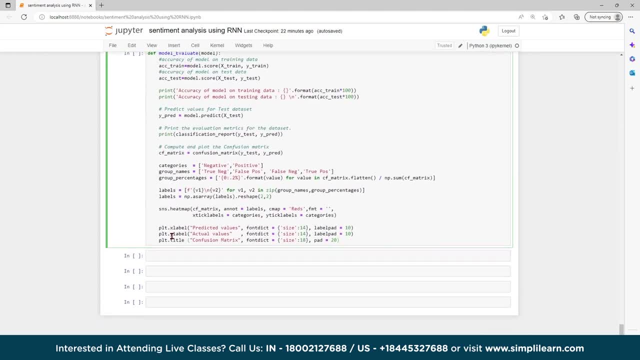 negative and the false positive. okay, so is nothing. that's, let's run it now. what we will do, we will do first for the logistic regression. so here I will write: LG goes to logistic regression. okay, then history was so: LG dot paid. explain: comma: white rain with a model. 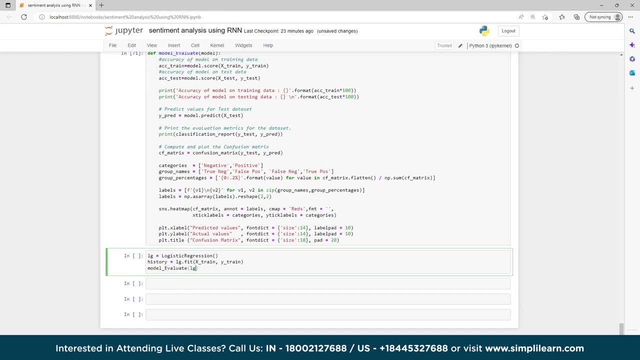 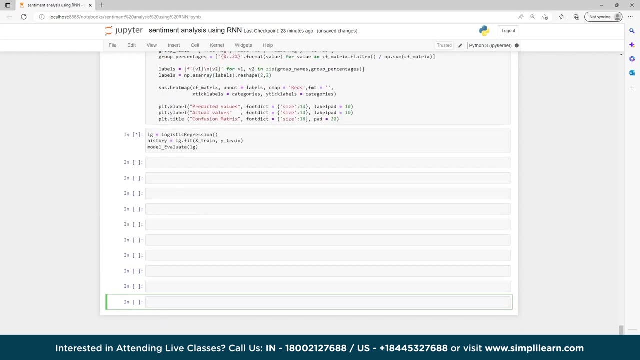 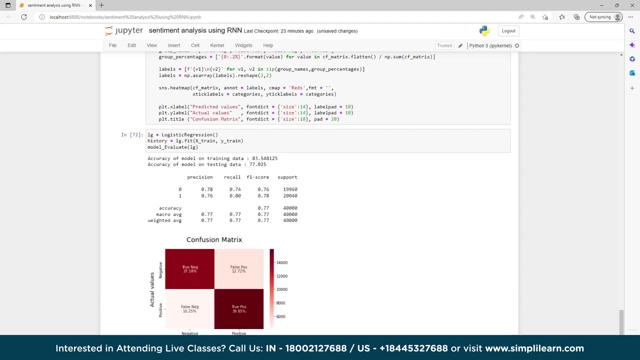 evaluate. I think. let's see, this is for the logistic regression. okay, see, the accuracy of the training deterred was enter testing the day some design parted? okay, you. this is the control matrix, the predictive value of logistic regression, and then the difficulty matrix, the predictive value of map law. Switzerland welcomes you as the solver of recipe forявiting your test of data behavior in terms of training data. that all percent, I understood. the training and personalization of the data. Falcon is, and it alpha large is actually all right. mathematical multitasking is of course necessary to solve here, only the 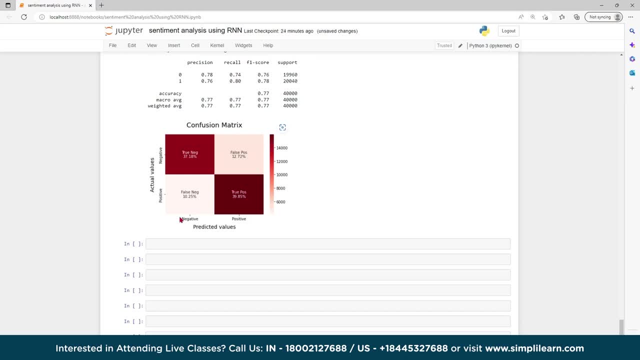 the predictive value. like these are the categories. now let's see for the linear SVM. for that I will write: SVM was to SVC and SVM dot fit rain, comma, white rain and model evaluate SVM. okay, and after that we will do for random forest and the new base. okay then. 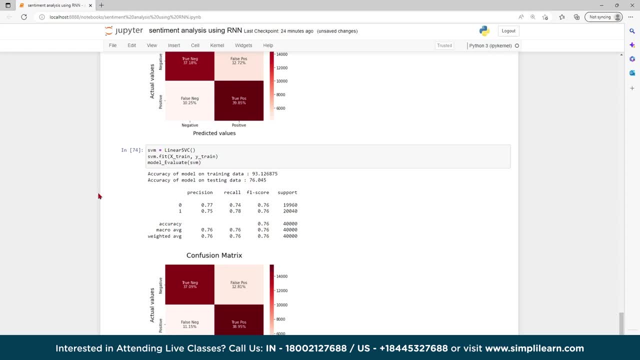 we will start with the RNN, so, as you can see the accuracy of the random forest and the new base. okay, then we will start with the RNN, so, as you can see, the accuracy of training data is very pretty good. ninety three percent and as if station. 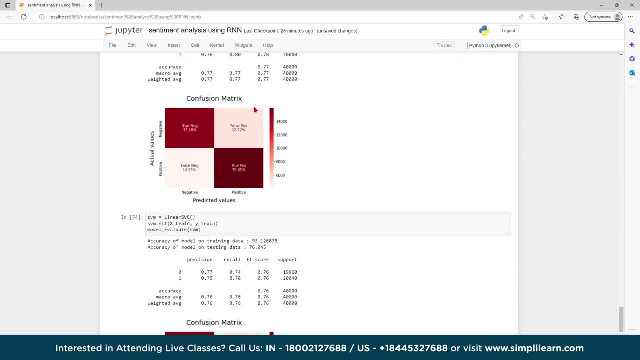 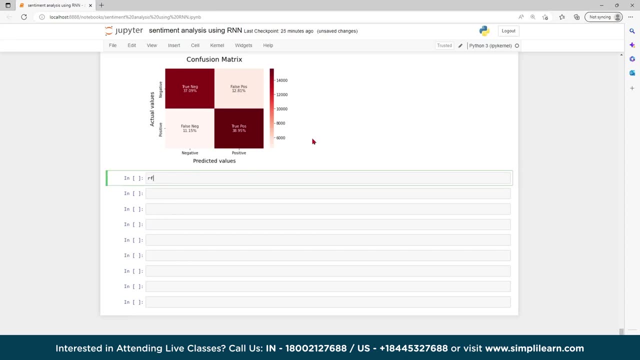 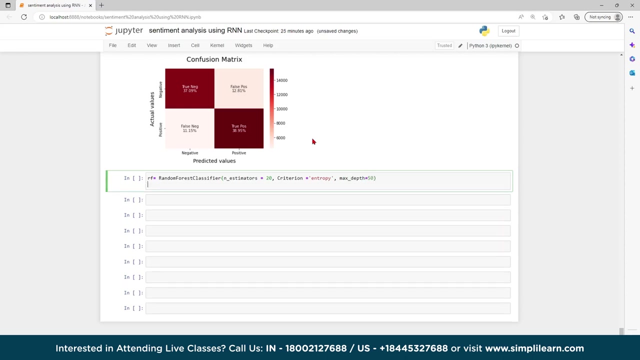 is eighty three percent and testing is less than regression model. let's see for the random forest. so I will write here RF because you random forest fire meters was to 20 and I did you on because to trophy more than max depth, question 50- then RF dot fit. 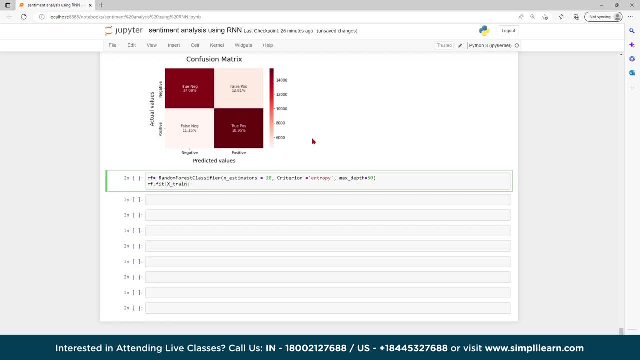 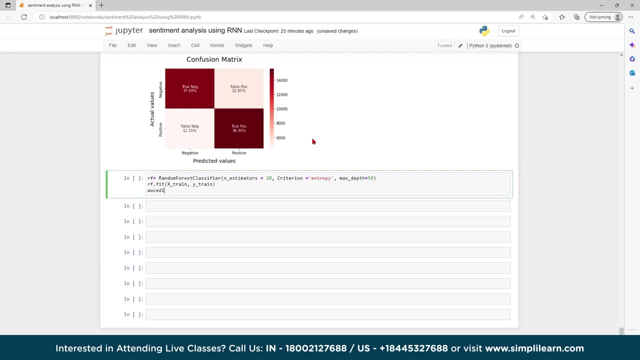 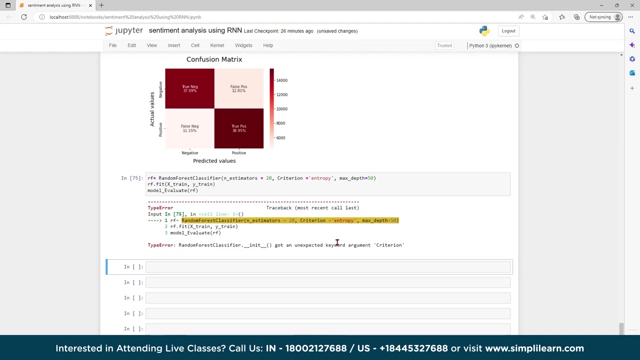 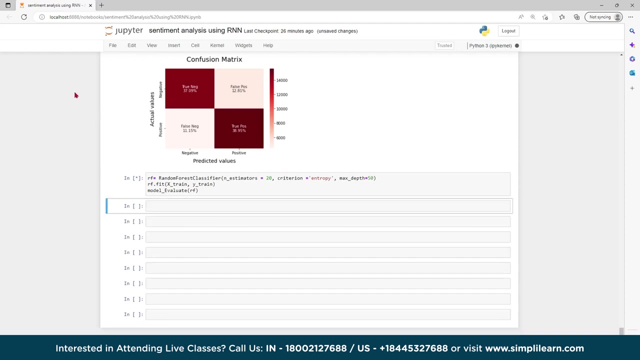 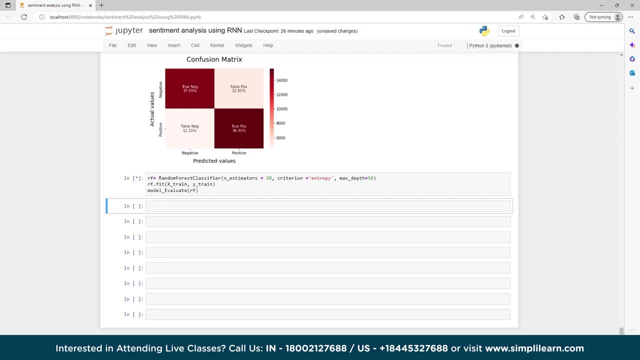 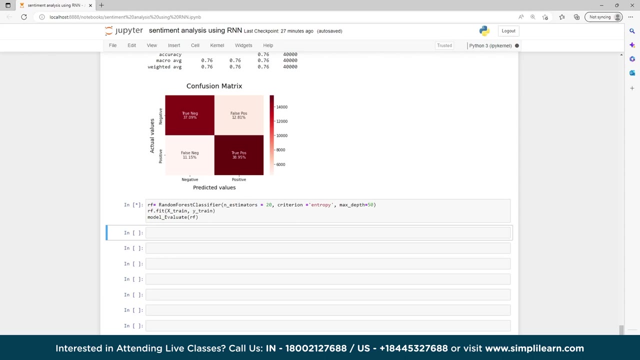 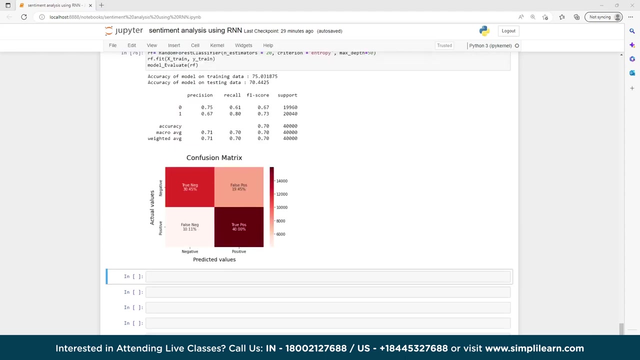 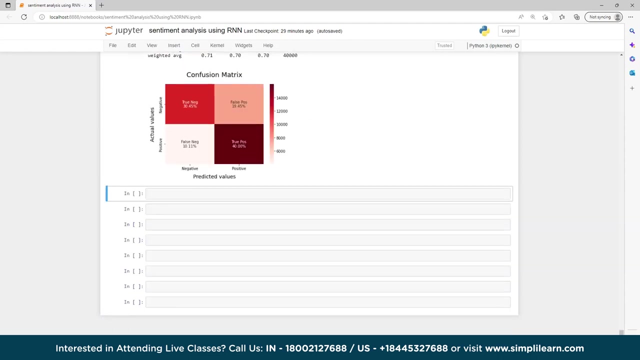 after this we will do for the name base and after that we will move on to them. our main model RNN- recurrent neural networks- still loading you, you, you will take little bit of time. so, as you can see, the confusion, matrix, so training, data accuracy: 75%, very less. so. now let's see the last model name base. 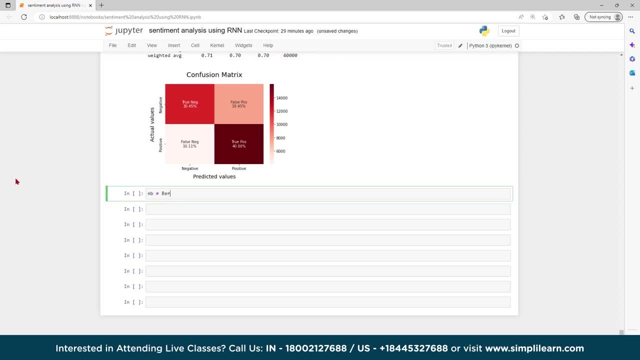 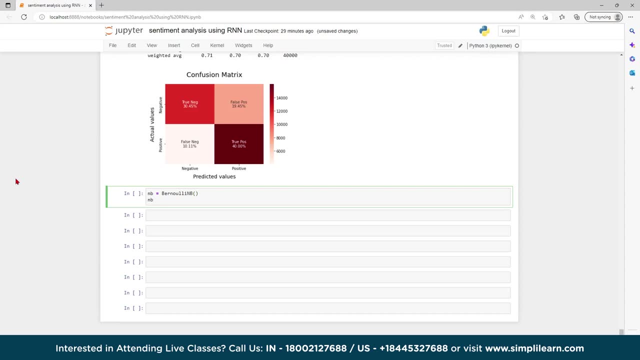 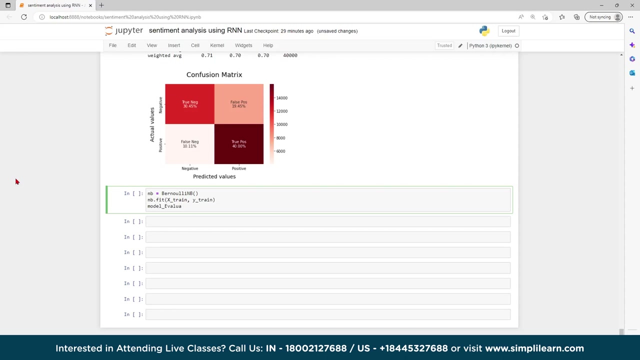 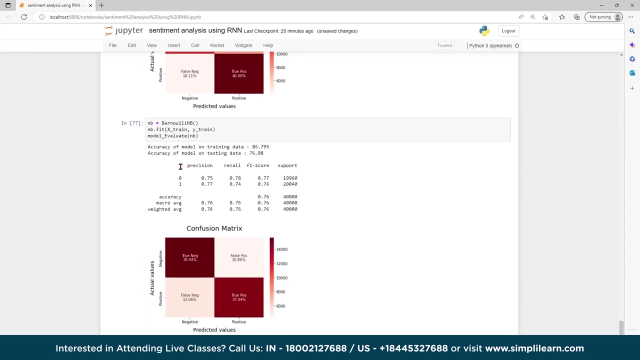 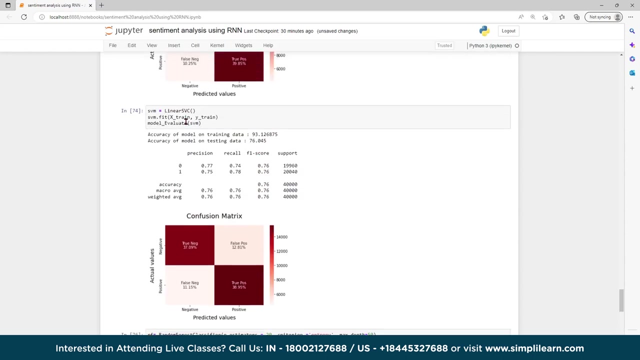 ok so, and be equal. so ok, so now we can be can be. ok, so now we can be: nb dot fed span comma, white rain. ok, ok, then model evaluate, then model evaluate. ok, then model evaluate. So Naive Bayes training 86,, 78, so as far, linear SCC has the best test training accuracy. 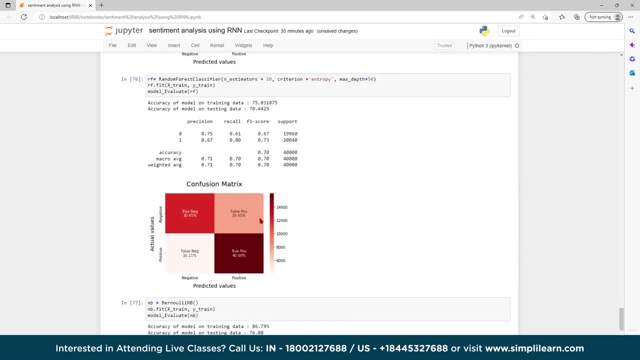 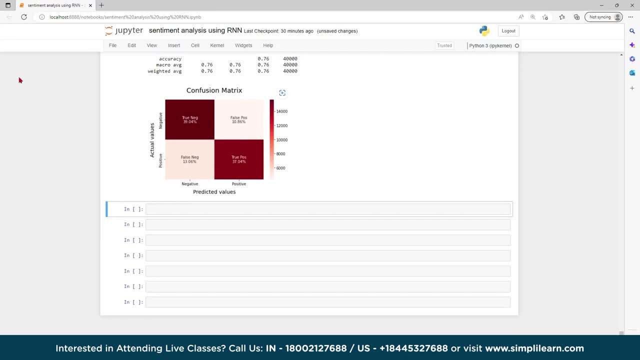 you can say: and the best testing accuracy is 76,, 70,, 76.45, see logistic variation. So now let's move to the our main model, RNN. So what is RNN, Recurrent Neural Network? at the start are the state of the art algorithm for sequential 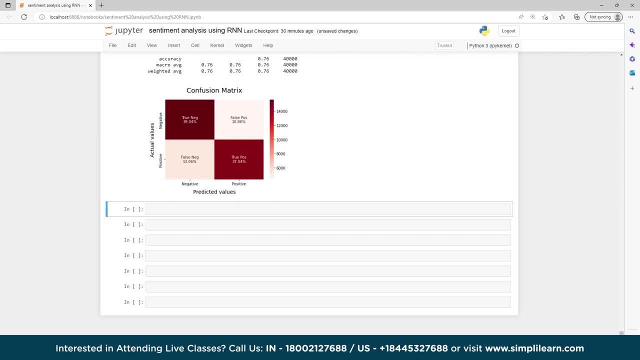 data and are used by Apple Siri and Google search voice. It is the first algorithm that remembers its input due to an internal memory, which make it perfectly suited for machine learning problem that involve sequential data. and there is one more thing: embedding layer. Embedding layer is one of the available layers in Keras. 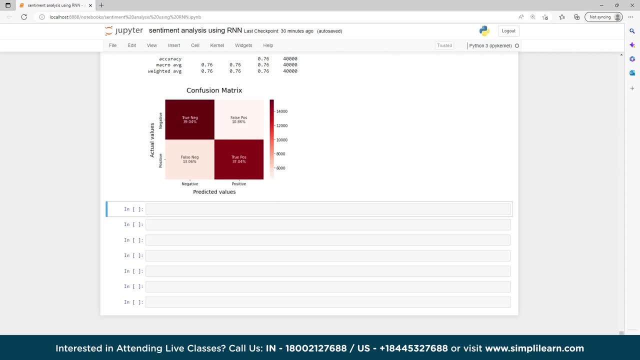 This is mainly used in natural language processing related applications, such as language modeling, but it can also be used with other tasks that involve neural networks. While dealing with NLP problems, we can use pre-trained word embedding such as GLOBE. Alternately, we can also train our own embeddings using Keras embedding layer. 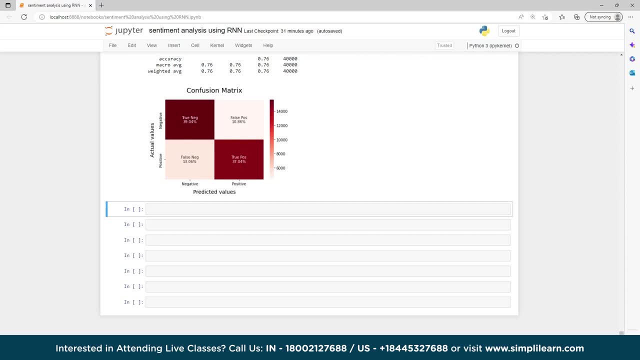 LSTM layer. Long Short Term Memory Networks, usually called LSTMs- I have made already many videos, You can check it out- were introduced by Skymetal. These have widely been used for speech recognition, language processing, sentiment analysis and text prediction. 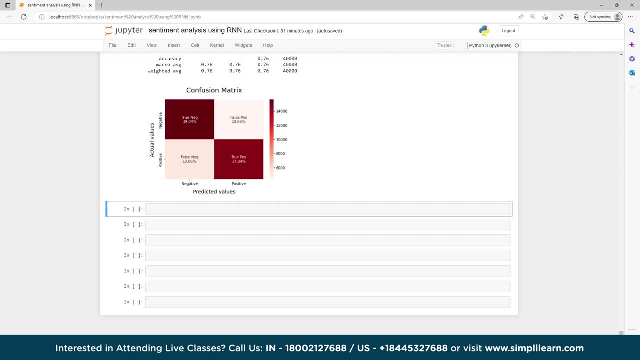 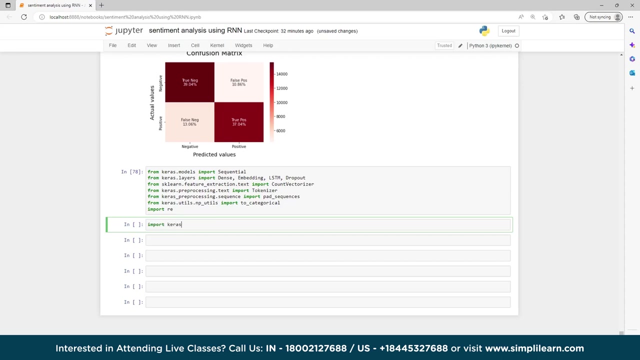 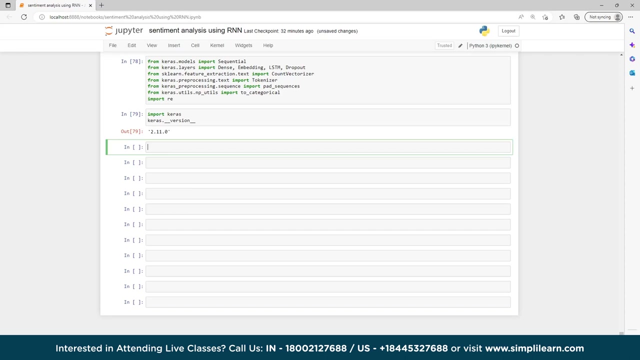 If you're going deep into LSTM, we should first understand the need of LSTM, which can be explained by the drawback of practical use of RNN. So let's start with RNN. Okay so here I will importing some libraries. Okay, So after that I will write: import Keras version 2.110, okay, fine, let's do that. 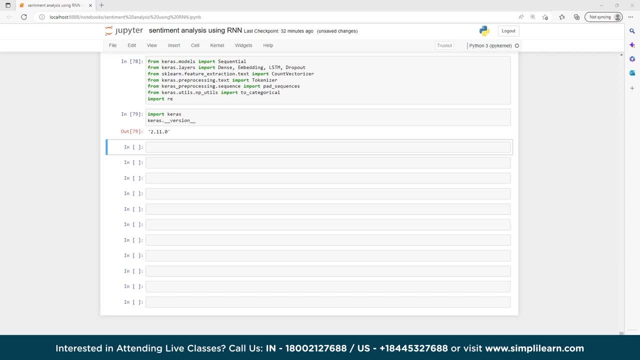 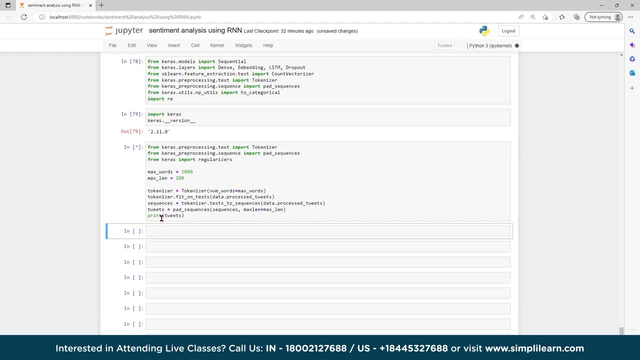 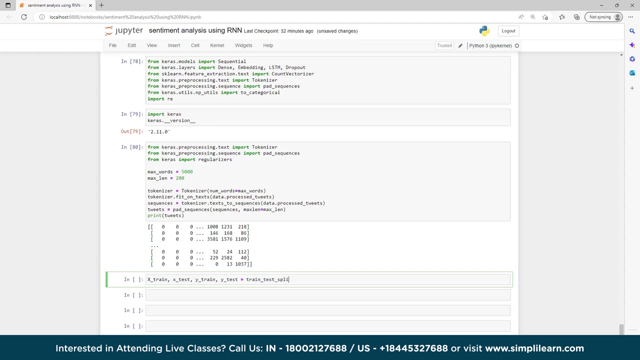 So now let's print: Okay, Okay, Okay, Let's test it. Test Sci, nicht io. train Test NEW LISTEN TO TRAIN TEST SIT. ORDER tweets: comma, data, dot. polarity, dot values. then test size was to 0.2. test size 0.2 means. 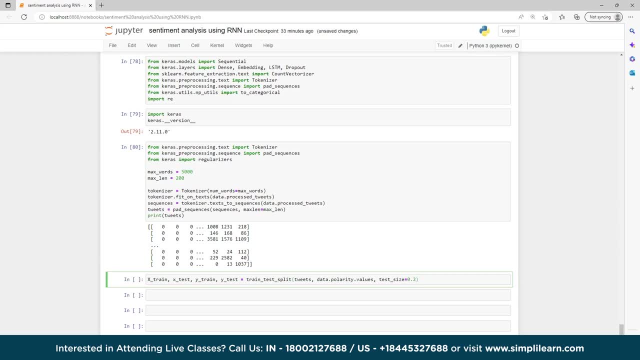 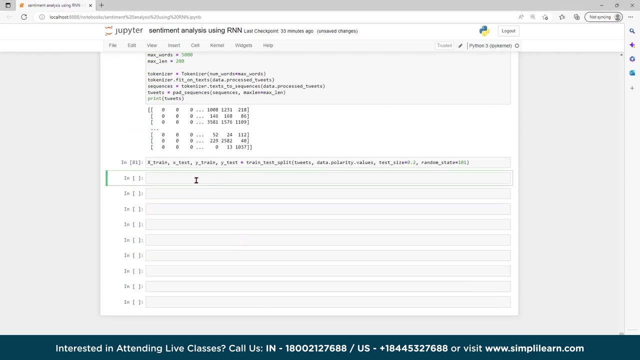 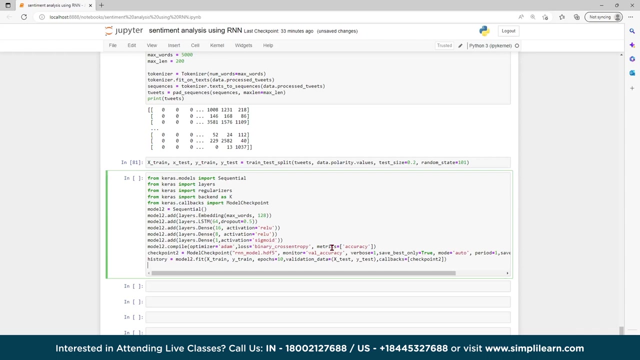 like 80 and 20 percent thing: 80 to training and then 20 percent to testing. okay, and let's the model evaluation. okay, so i will. these are relu signals, all the you know the layers. so now this epoch, it will run till 5000, like. 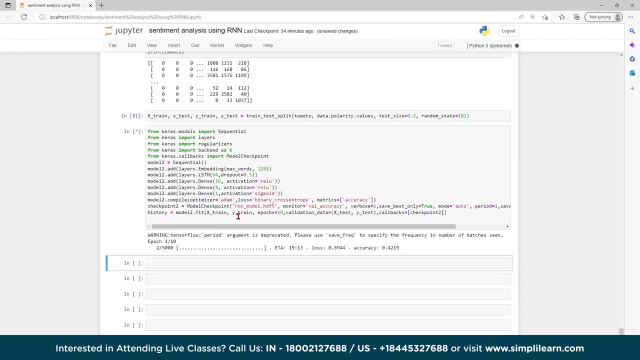 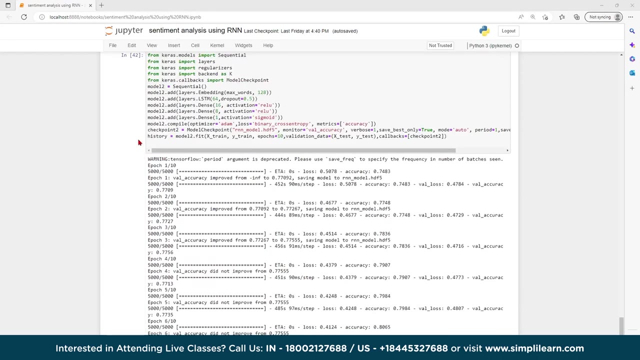 count will go till 5000- okay, see the 5000- and it will go to 1 to 10. so it will take time, so i will get back to you after this, completing this. okay now, as you can see the epochs then successfully. okay, so what should i do? 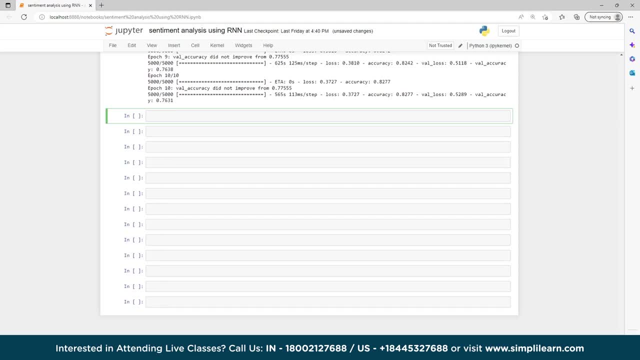 but i will give some space here. oh, now we will see the positive and negative outcome. okay, this is something like testing. okay, we will test, we will predict, we will give one uh, a sentence and then we will predict it is coming right or wrong. the accuracy is giving a right or? 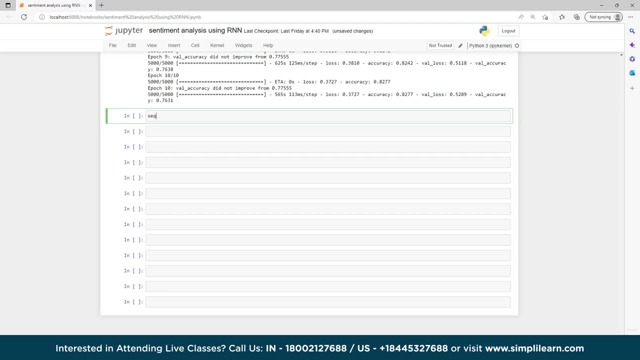 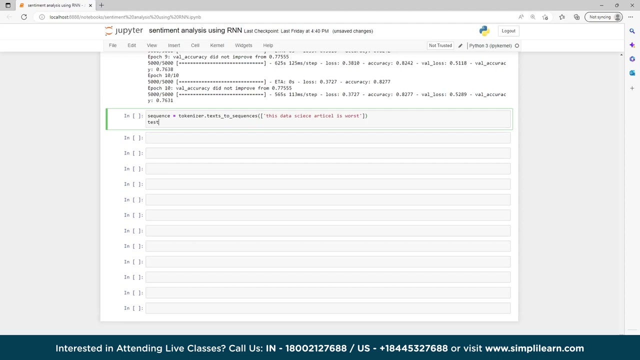 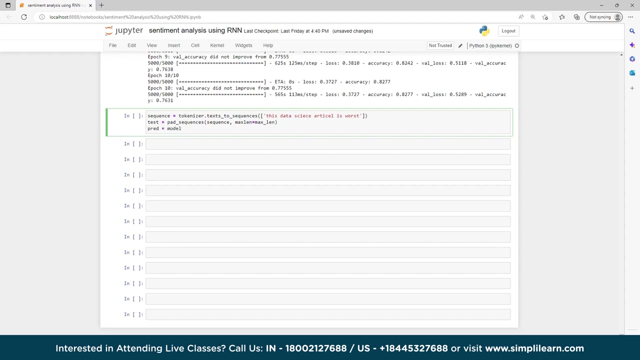 wrong. okay. so here i will write: sequence equal to tokenizer dot text to sequences. then I'll write: this data science article: this worst. okay. so here I will write: test equals to bad sequences. and here I will write: sequence: max length was to max length. then I will write here: prediction equals to model. 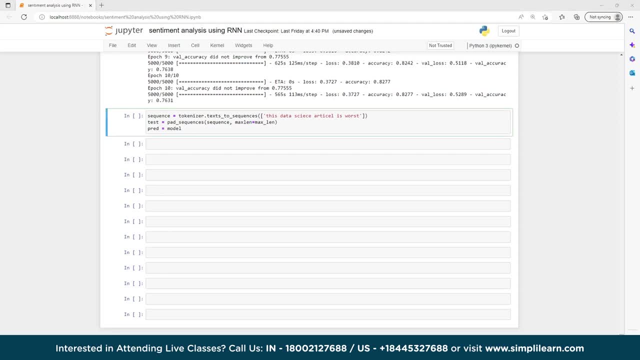 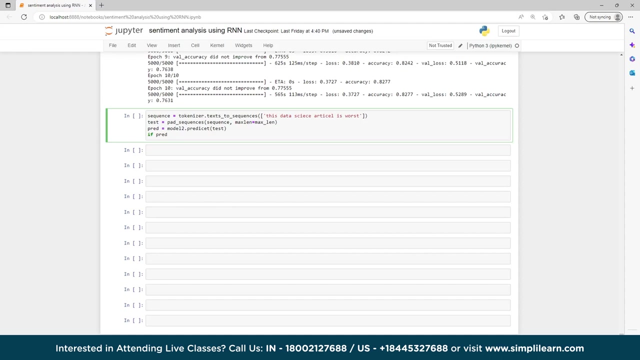 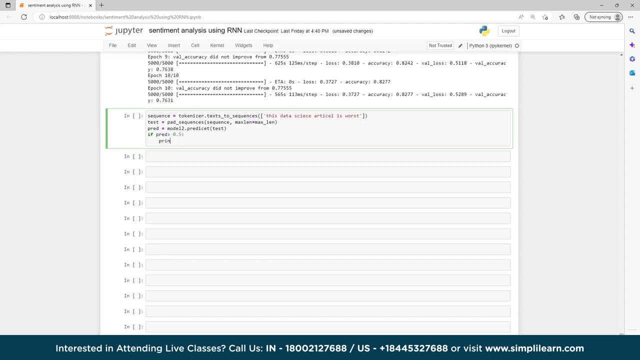 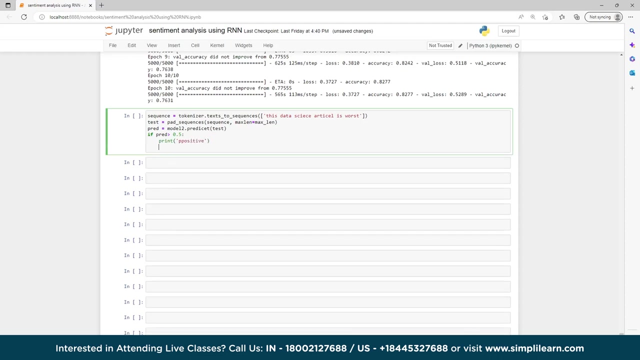 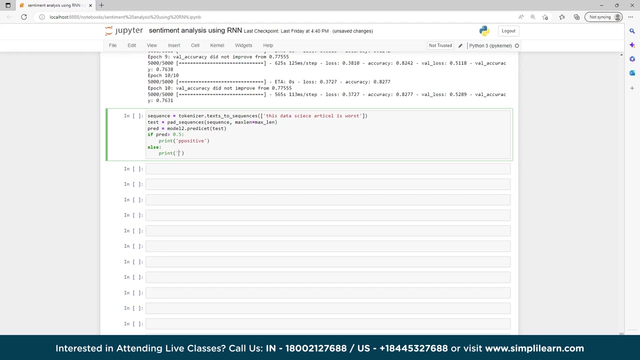 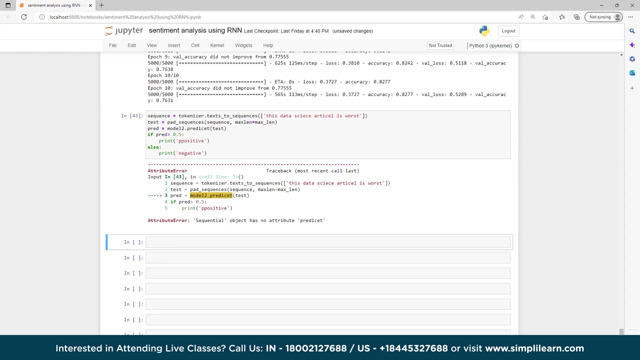 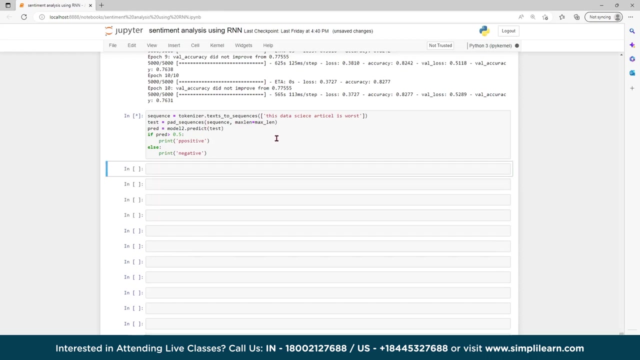 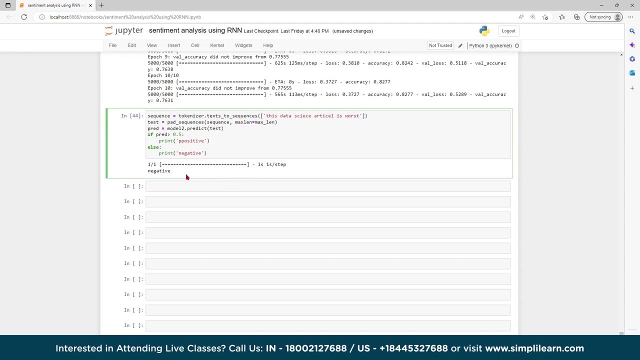 right model, then write model 12. two dot predict, then test, test. okay, if diction is greater than 0.5 means 50%, then it should print positive, it else negative on this sequential object has no Cause. it is the word worst is showing correct. 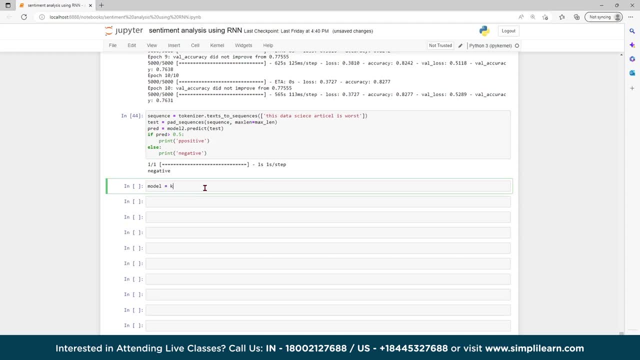 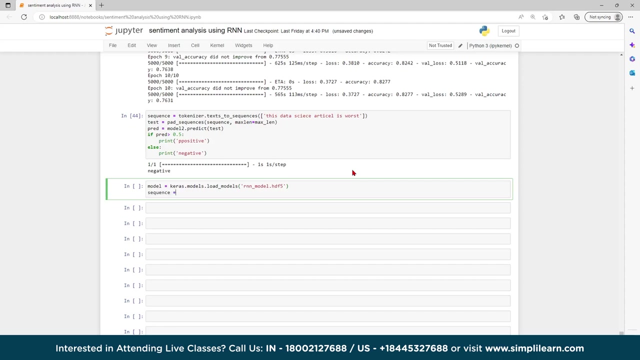 Check from the RNN models. model equals to keras modelsloadModelsекст. here we will load RNN model, rnn underscore model dot: sg f5. it is pre-trained model. okay, pre-trained rnn model. so sequence pursue tokenizer dot text to sequences. then I will write here: 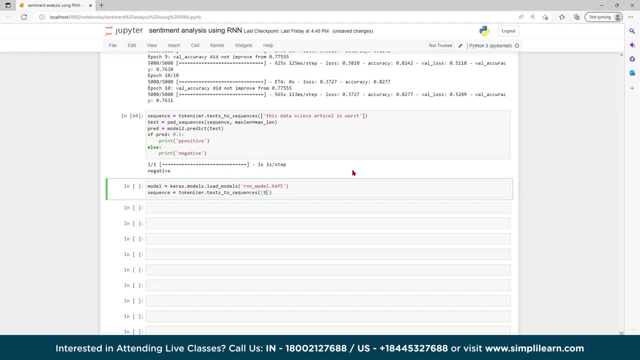 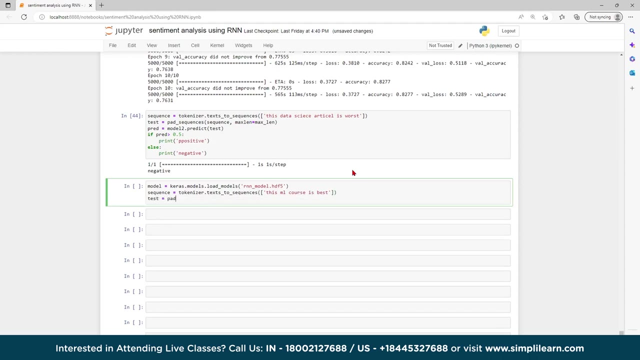 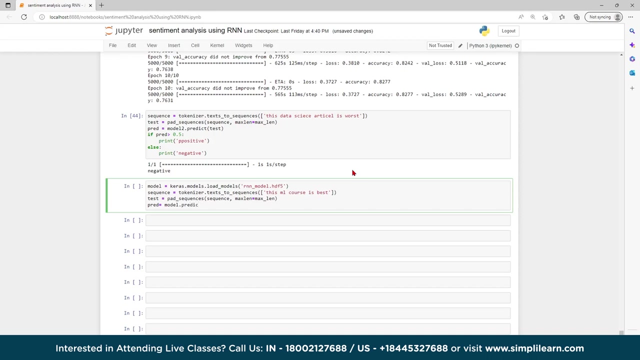 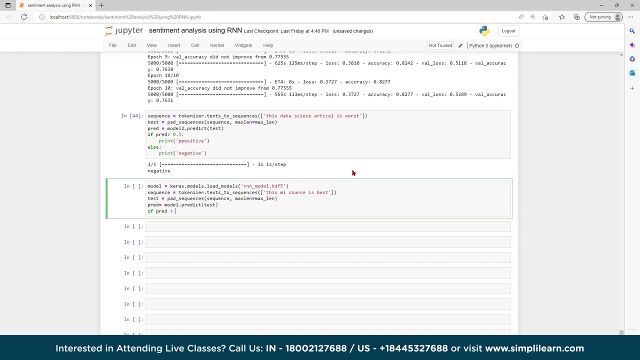 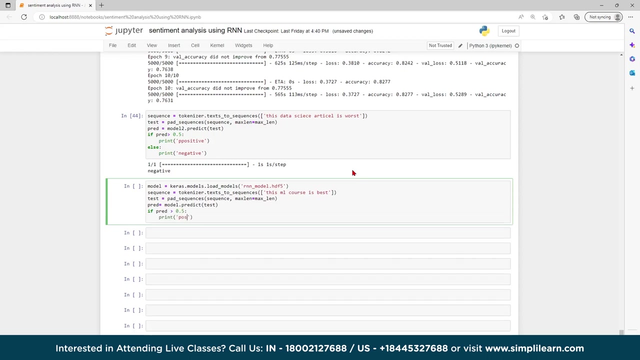 this, this ml goes, is best. okay, best equals to pad underscore sequences. sequence equals length, length, length underscore length. then prediction equals to model dot. predict then test. if prediction is greater than 0.5. 0.5, then positive. 0.5 means 50%. 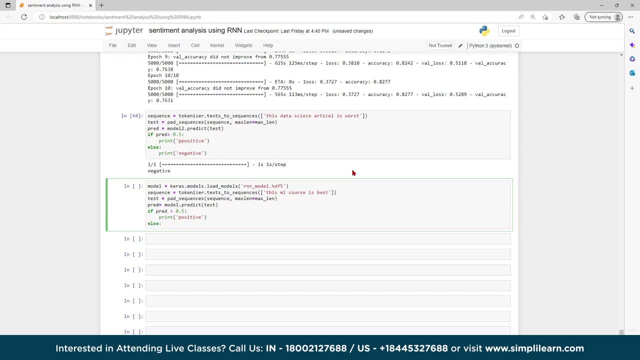 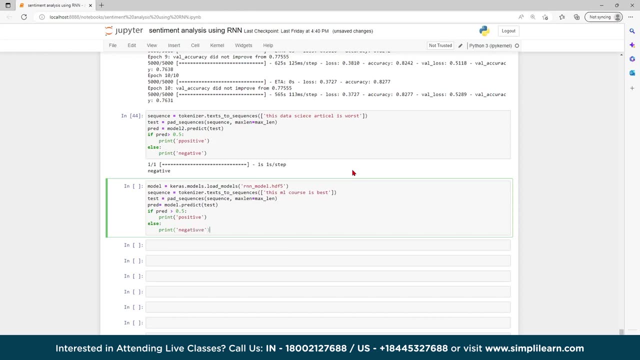 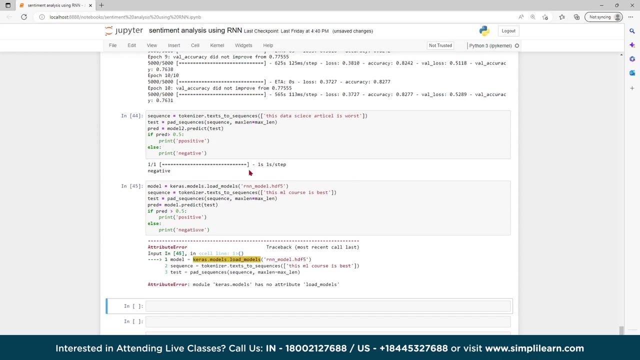 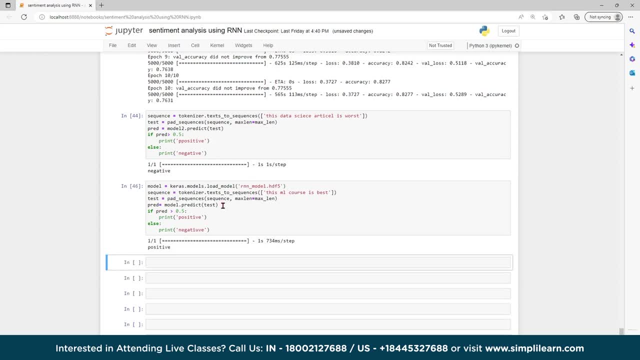 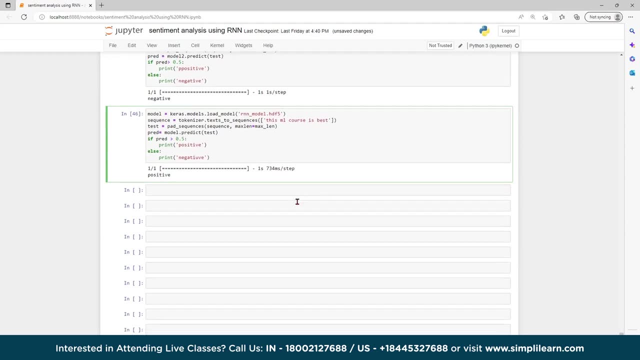 0.5, 0.5, 0.5, 0.5, 0.5, 0.5 course is best, so there is no negative word. okay, so what we will do now? we will do model saving, loading and prediction. okay, so for that I will write import pickle while it was open. 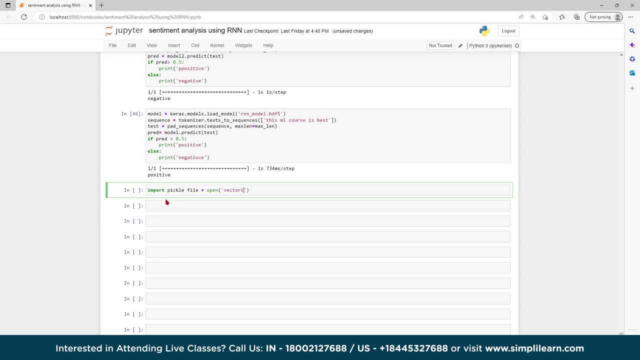 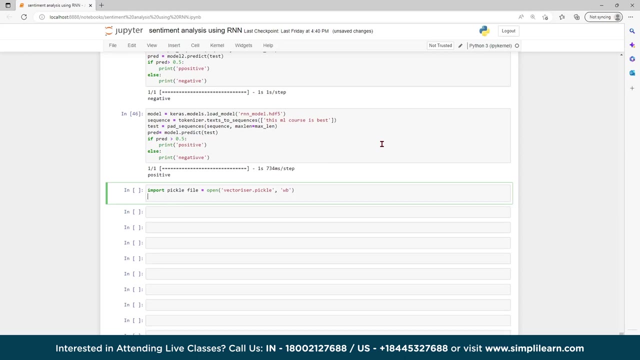 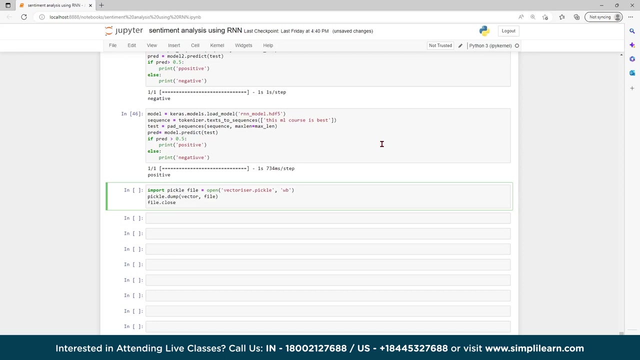 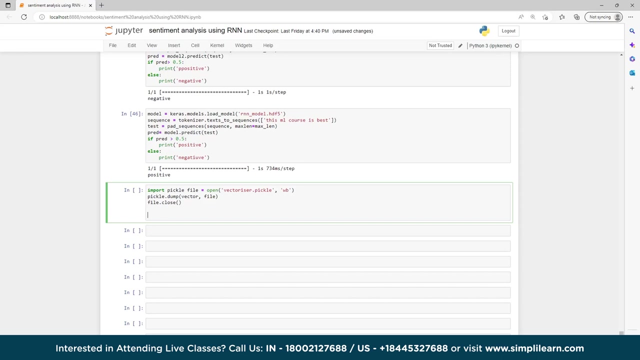 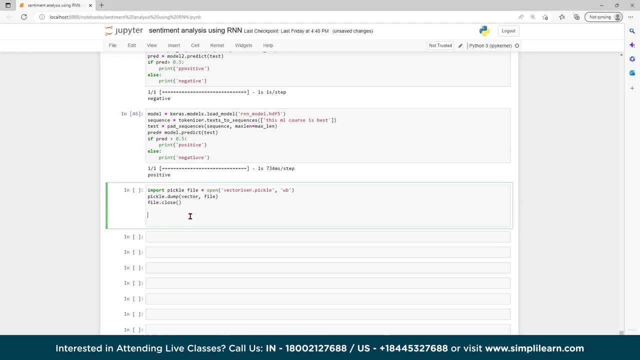 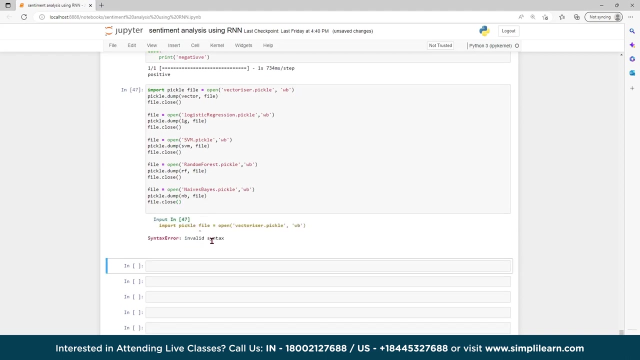 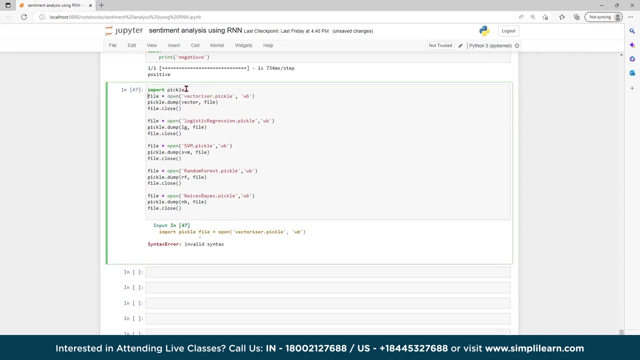 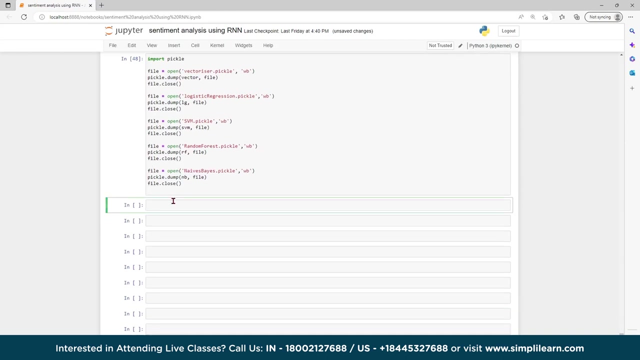 vectorizer pickle and wb pickle, and here I will write pickle dump, dump, vector5, vector close. okay. so like this, I have to write for name: base, logistic regression, svm and random forest. so what I will do right here. okay, let's run this. okay, now what we have to do. we have to: 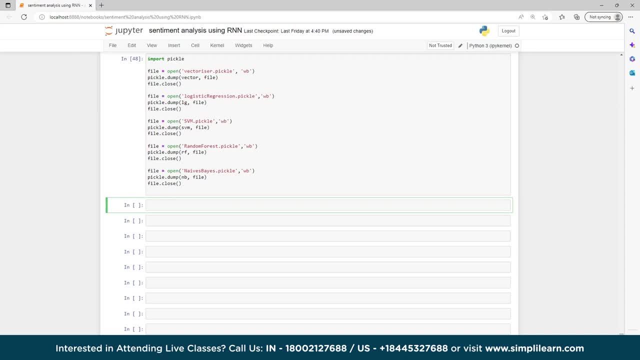 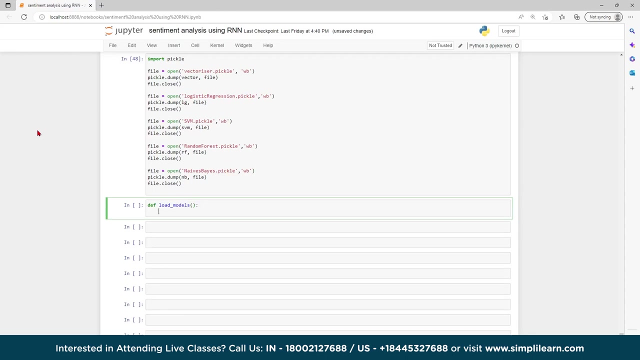 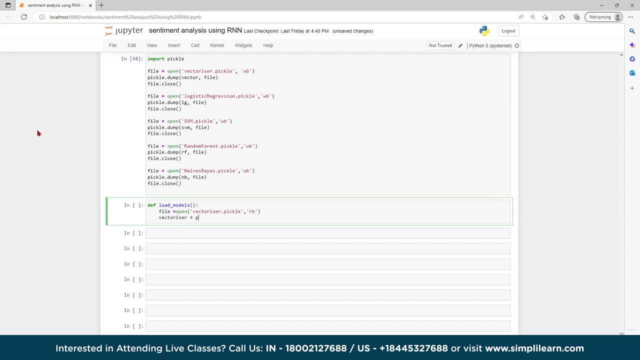 predict using saved model. okay, what we will do here: we will load model first and we will predict. okay, so first I will write the function name- load models- and we will load the vectorizer. so file equals to open vectorizer pickle rb and vectorizer pickle. 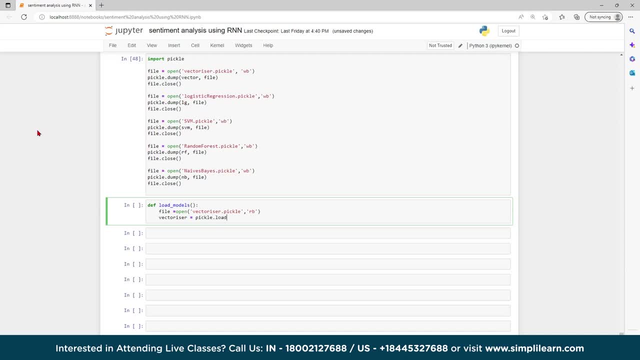 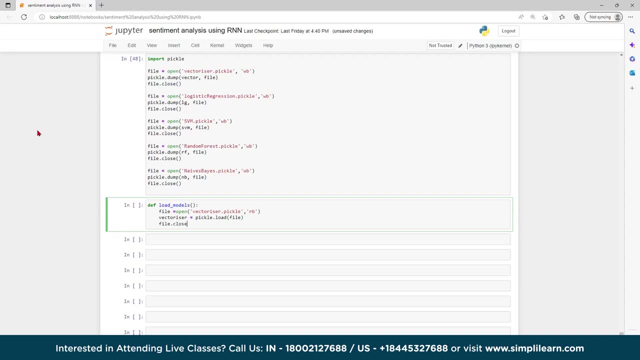 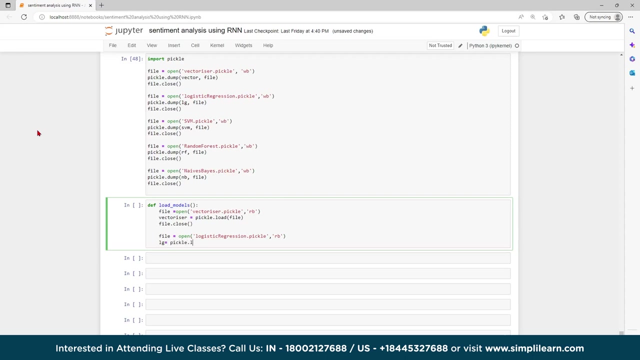 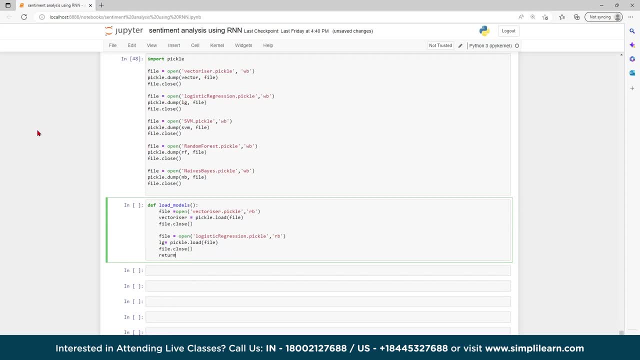 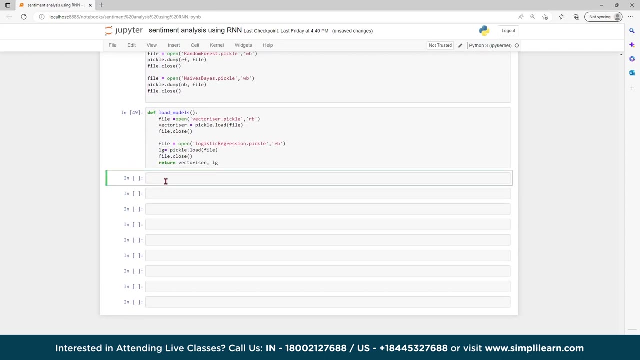 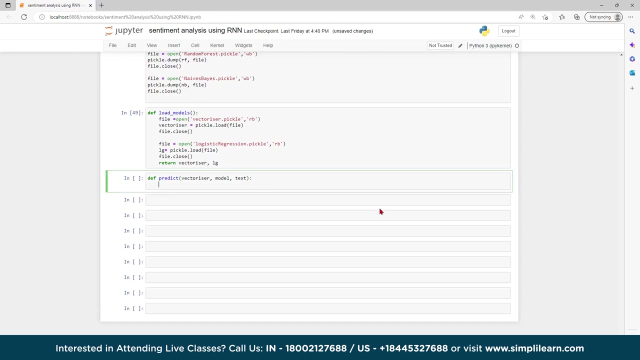 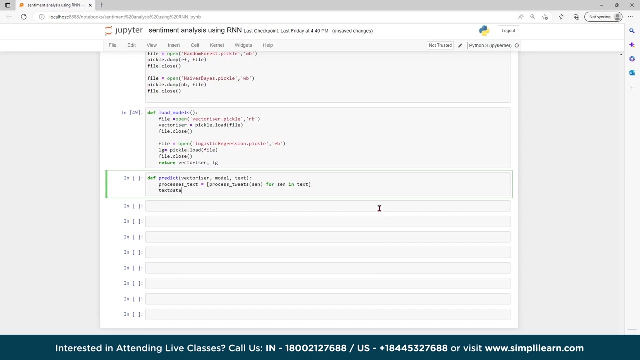 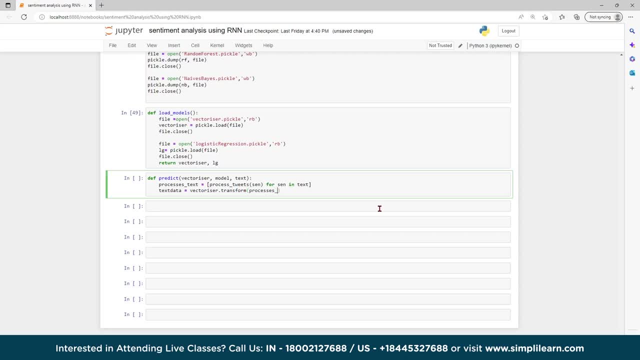 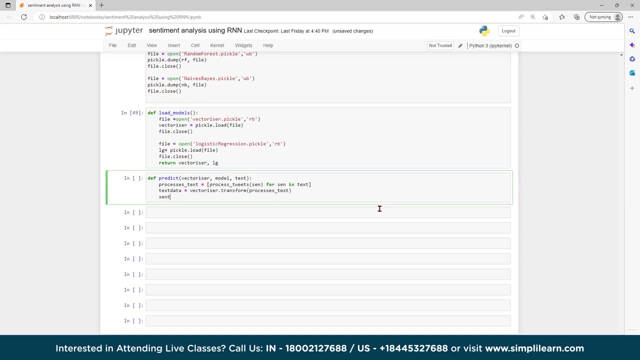 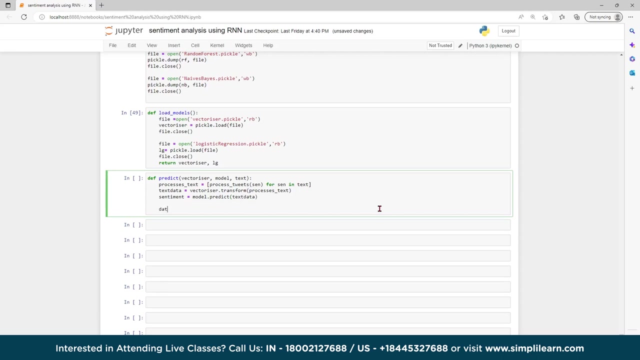 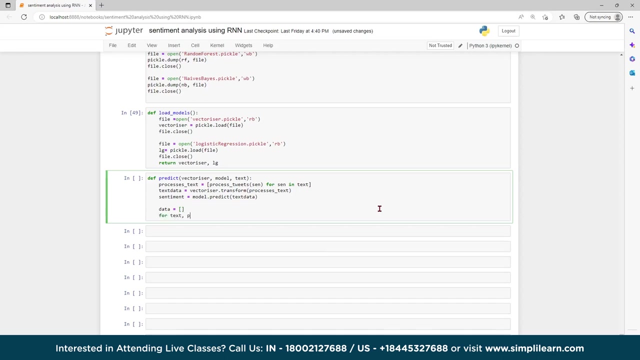 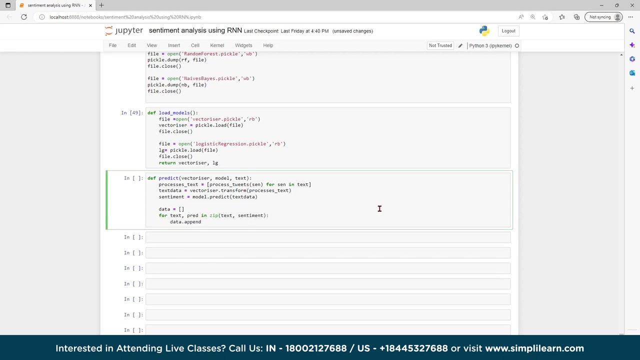 this is then sentiment model: dot predict. so here I will make a list of text with sentiment. so for that I will let data equals to empty array. then for text prediction and zip text comma: sentiment data dot. append text comma: prediction. okay, 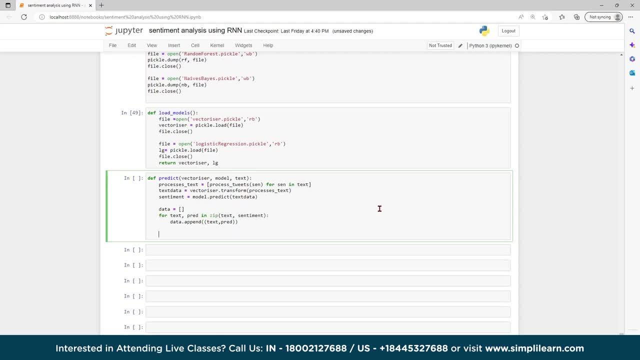 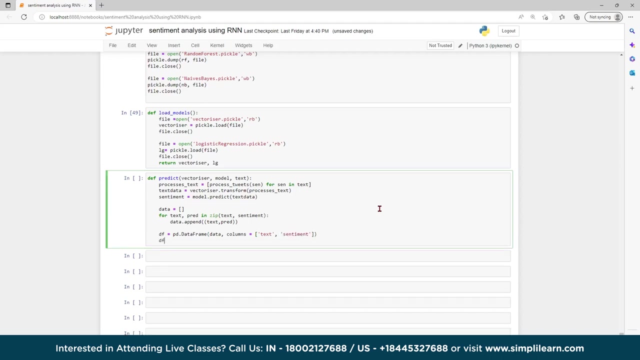 then we will convert the list into pandas data frames. so for that I will let df equals to pd dot data frame data comma, columns, person, text, comma, sentiment. okay, then df equals to df dot. replace: okay then percentiku comma. one negative comma positive. 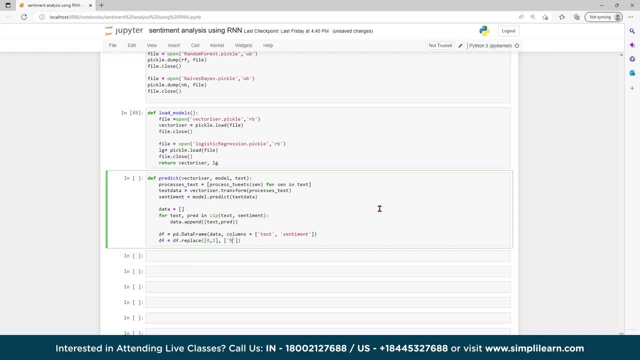 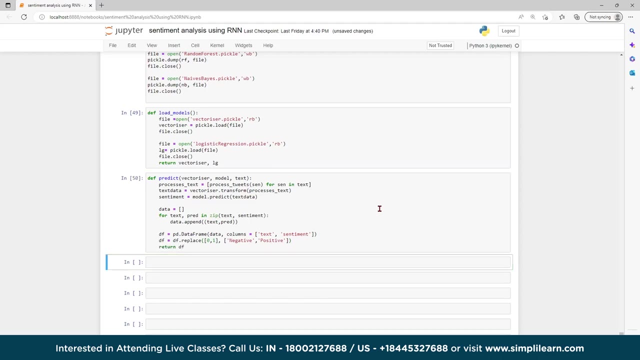 And here, okay, And so at last I will write: here isn husband not5, not6,, not7, not8, dac. we will and we will end in only this: n2 to and 8 to- group. 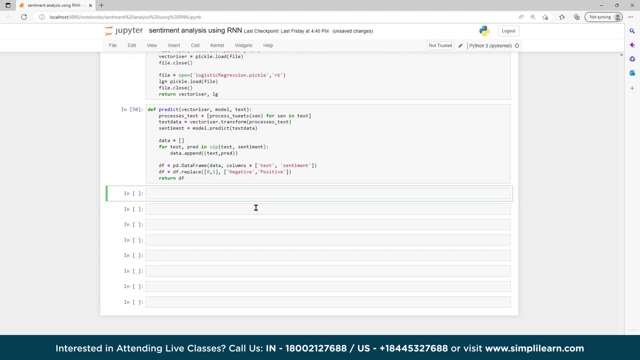 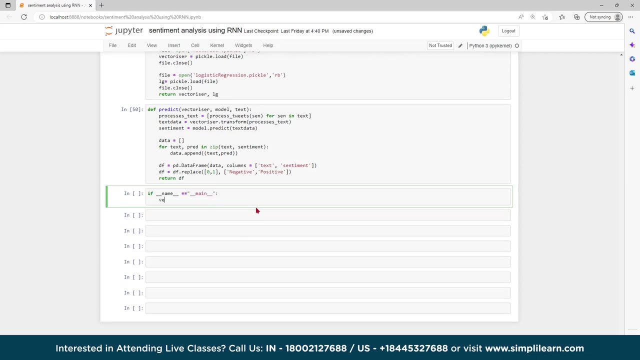 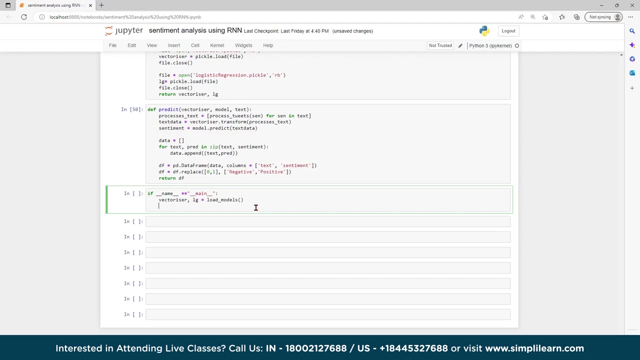 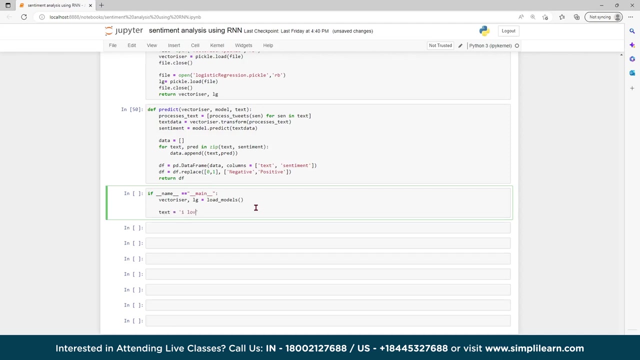 There we go. So that's it. Yeah, perfect. Thank you for playing. I appreciate the question and here we will loading the model, here we text to classify, like what should be in the list. so like text and I will like, I love machine. 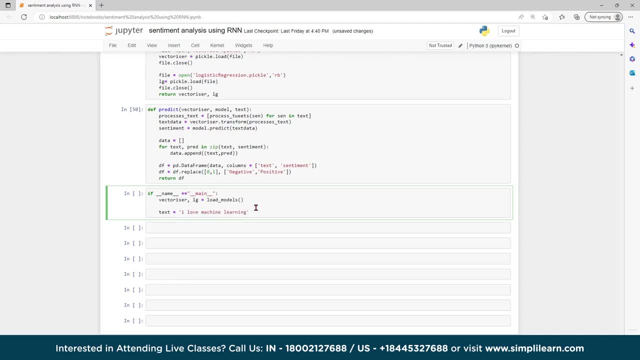 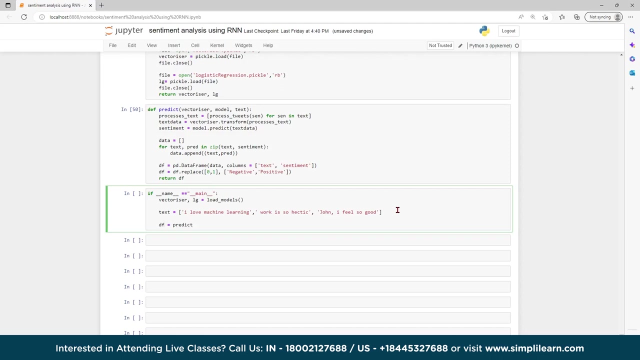 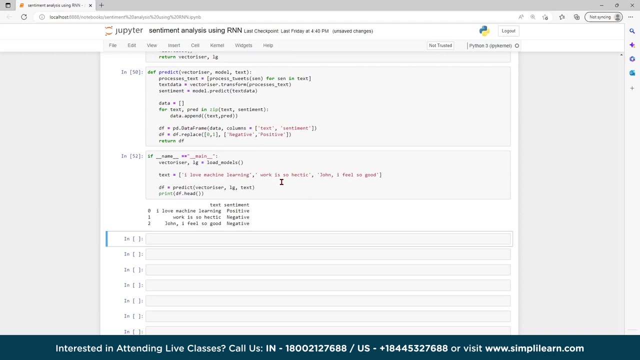 so let us go to the the field. so here: df, so date. try that command. here we can display the code, the c, eco, so Text. then print dfnet. See, I love machine learning. positive Work is so active, positive, Turn off, feel so good, negative.